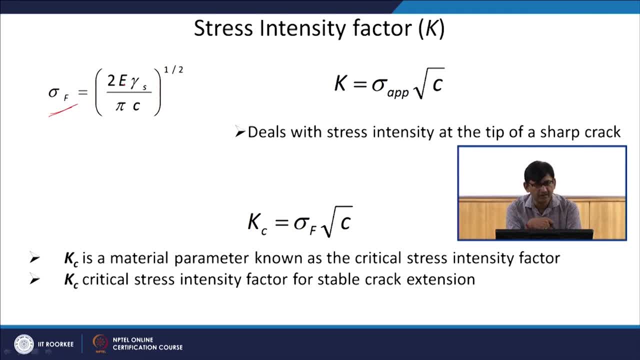 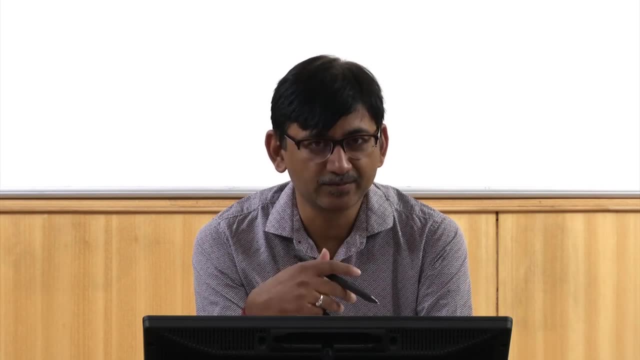 there will be some plastic deformation ahead of the crack. this actually stress will be more, while we are talking about ductile material, That means you will need more stress to continue the crack or propagate the crack. okay, So it is always better to design your material or your you. whatever you are the structure. 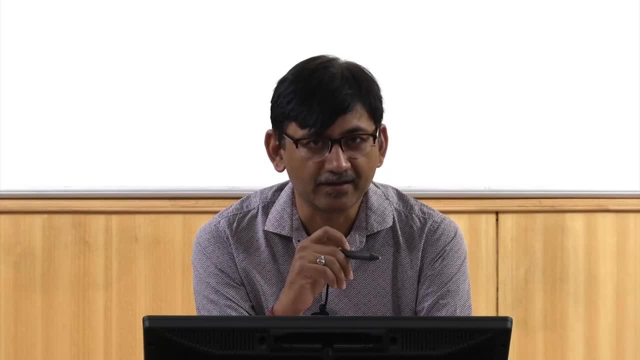 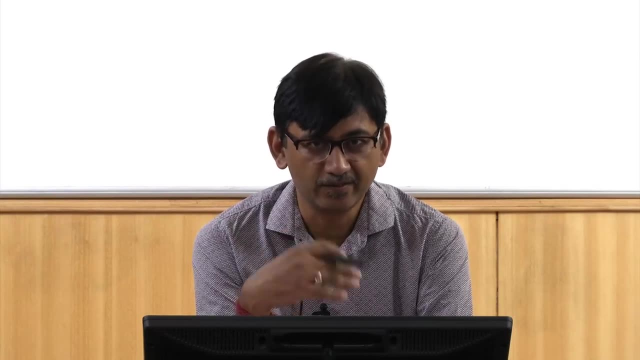 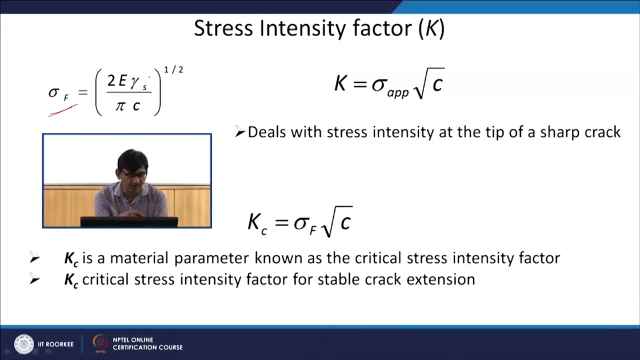 you are designing, considering only the, considering it as a bitter, brittle material, so that you are always going to give a conservative estimate. okay, You will be always within the safe limit, okay. Now the problem with the Griffith equation here is that you have a parameter which is the surface energy, okay, the gamma s and it. 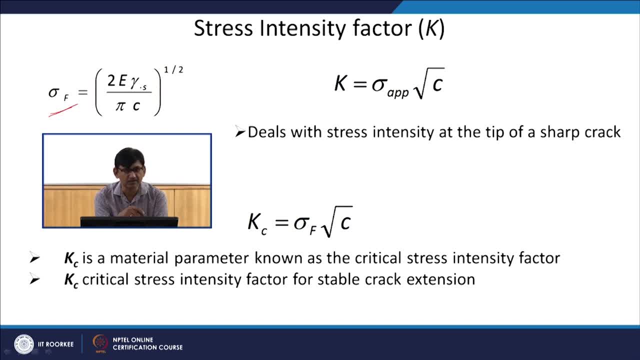 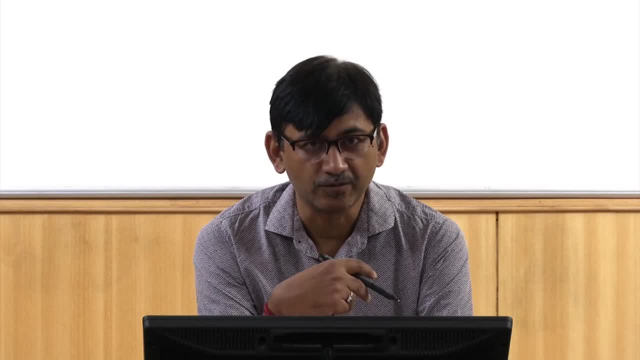 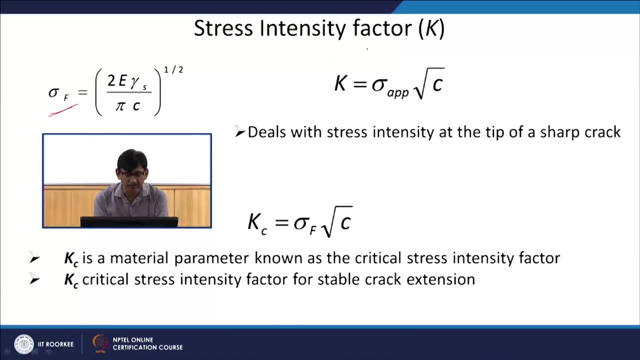 is very difficult to kind of find out this. in all kinds of material, if you change the composition, these energies will change. okay. So for each material, finding out this energy is always going to be difficult, okay. So instead of that, another proposed idea is that 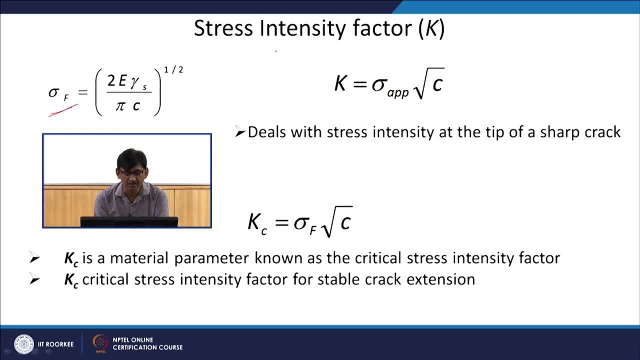 we can calculate a parameter, Coulomb, called stress intensity factor. okay, and what stress intensity factor says? that K is dependent on the whatever is your applied stress under root of the crack length. okay, So if it is a, the crack within the material, it will be 2, the total will be 2C. okay, so, 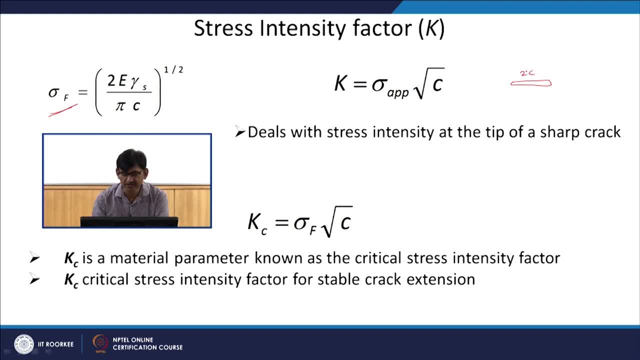 half of that for inside crack. if it is edge crack already, we will take the total length as C, so it deals with the stress intensity at the deep of a sharp crack. okay, Now you can also define a critical intensity factor in this. okay, so this will be when. 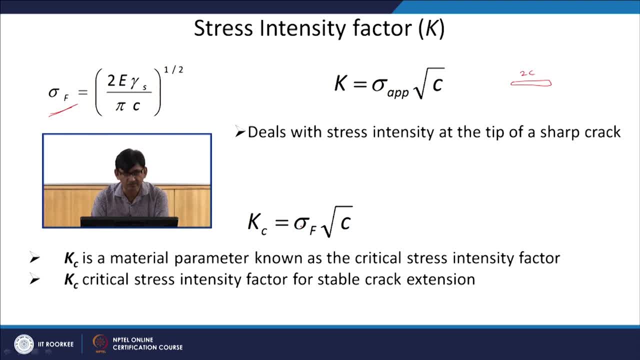 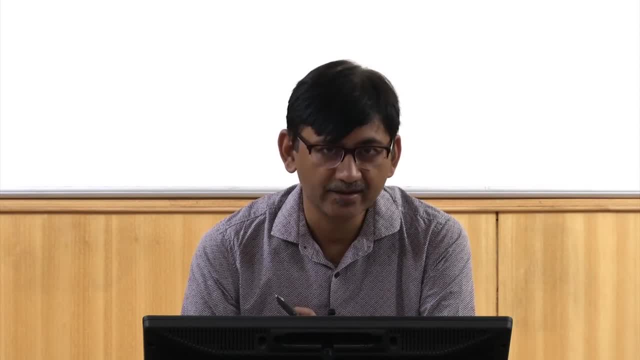 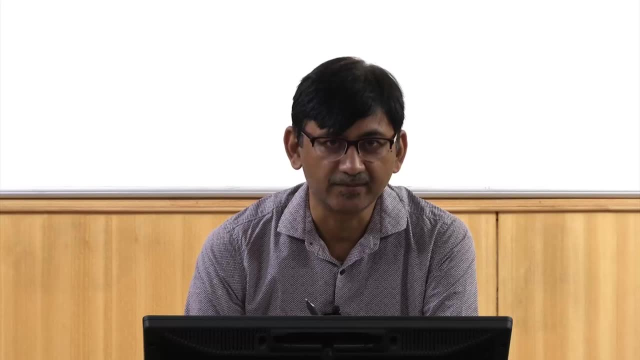 the stress is sufficient to start the fracture, so it is sufficient to start the crack propagation. so, as Griffith criterion has already assumed that we believe that there are going to be small defects, Cracks inside the material, okay, so when the material fractures, basically these cracks, 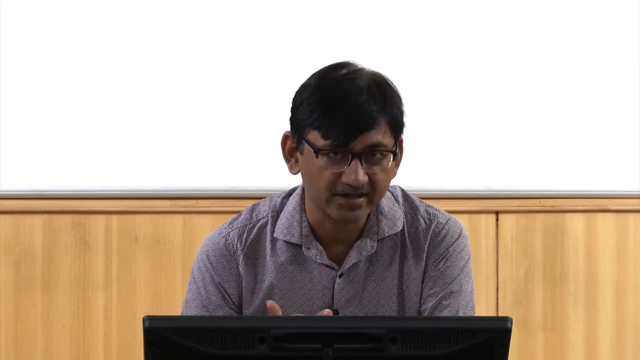 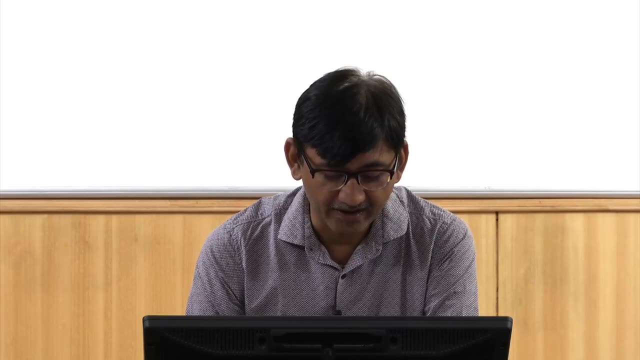 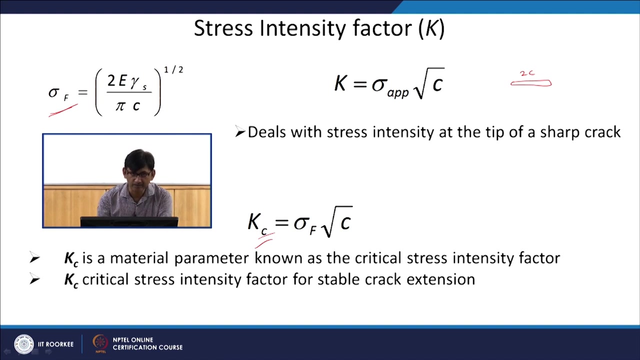 are going to propagate, okay, so we want to find out a stress, okay, which is sufficient to propagate these cracks, and for that we can define critical intensity factor. okay, and with that will be. now we have removed, change the sigma applied to sigma F. that means: 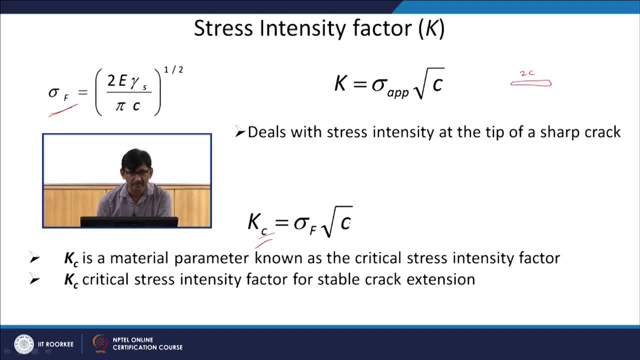 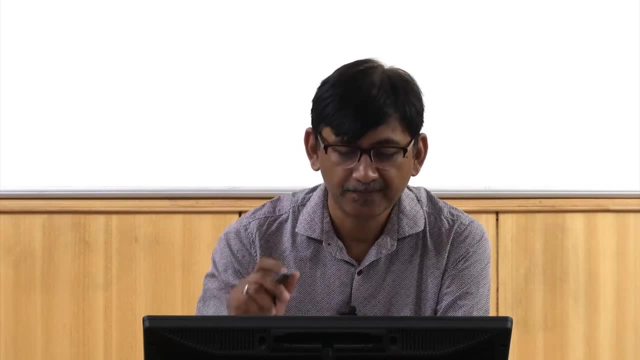 the stress where the fracture is going to take place. okay, And this is again the crack length. so this is Kc is critical stress intensity for a factor for stable crack extension. okay, So instead of doing this analysis using surface energy, we can do an analysis like this and: 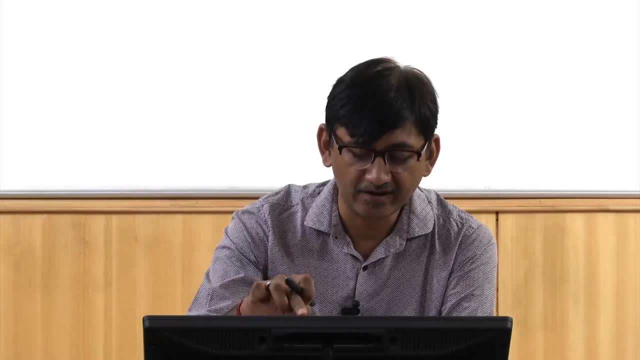 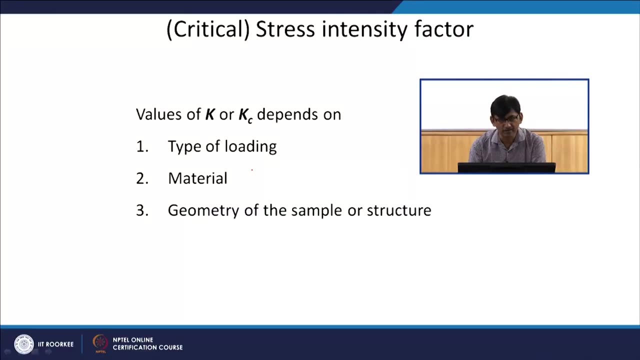 we can find out the critical intensity factor for a given material. okay, So your value of K or Kc will depend on type of loading, what type of loading I am giving material. Okay, So for each material, I can find out the stress intensity factor, critical intensity factor. 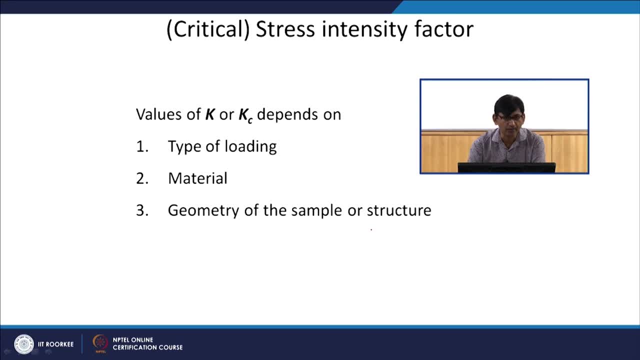 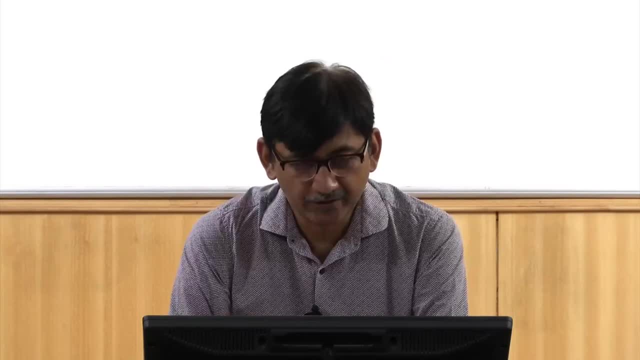 and geometry of the sample or structure. okay, So what is the geometry of the structure? is there? okay, We will look into detail of all these 3 parameters. So the first one, if you see this, is a 3 modes of loading. okay, 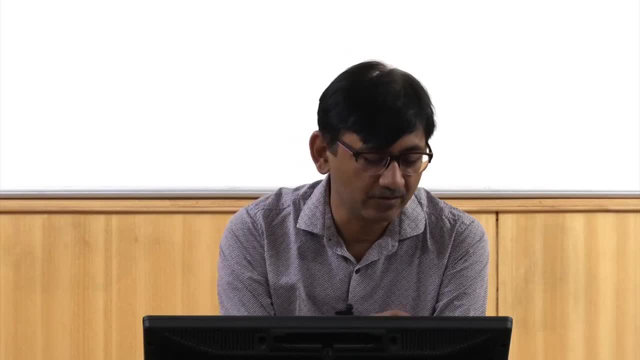 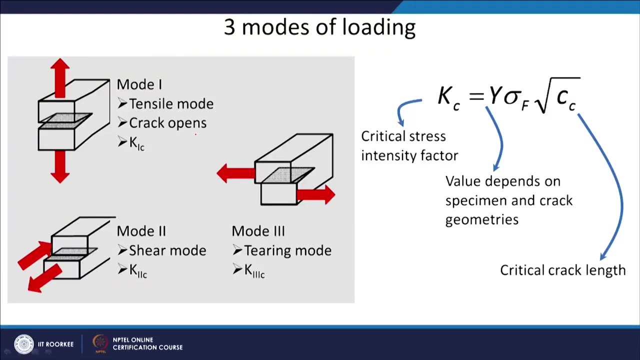 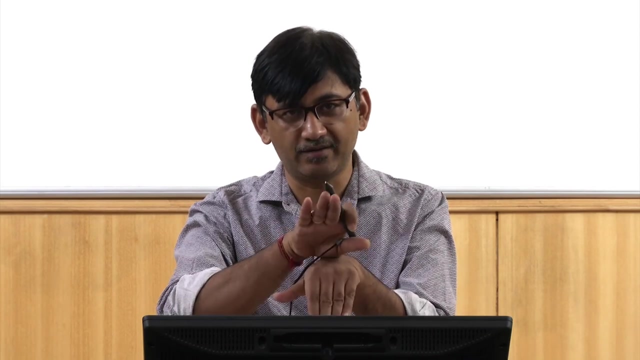 So mode 1 is what we call as tensile mode. okay, So if a edge crack is there and you are applying a tensile stress, Okay. So it is called a crack opening kind of mode. okay, So whatever crack is there, it is going to be opened by application of this tensile stress. 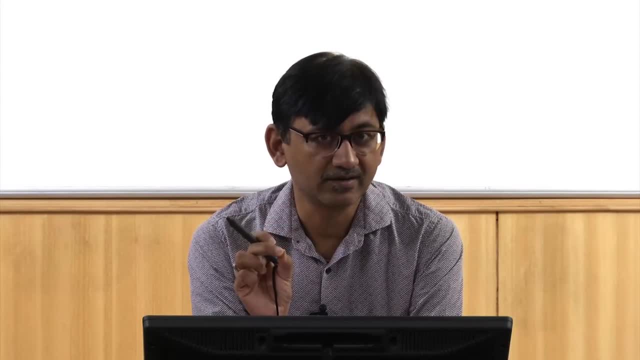 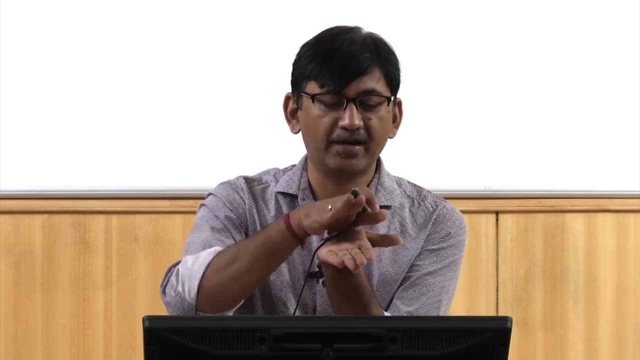 Just a comment here that compressive loads are not, the are not that critical in case of fracture. okay, Because when you are applying, suppose, there is a crack. also, when you are applying a compressive load, stress actually you are closing the crack, okay. 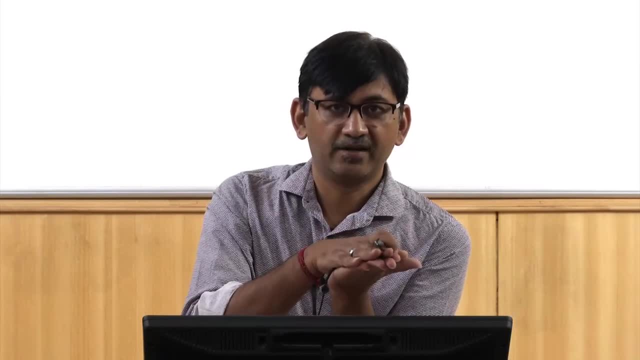 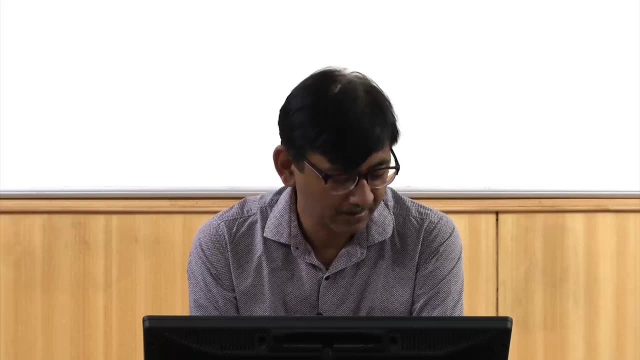 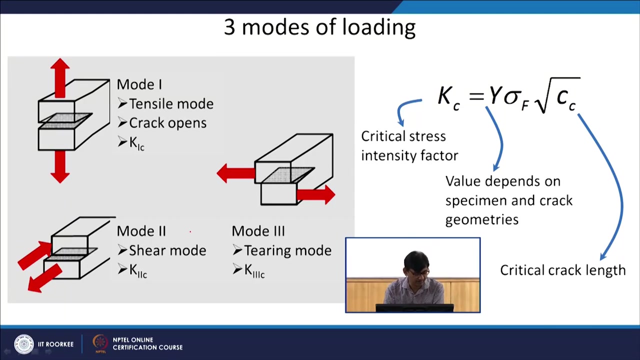 Okay, So it is not going to propagate, In tensile mode only it will propagate. That is why you will not see a compressive mode here, only a tensile mode. Then the second mode is the shear mode. okay, So basically I am shearing the material where the crack is there. okay, 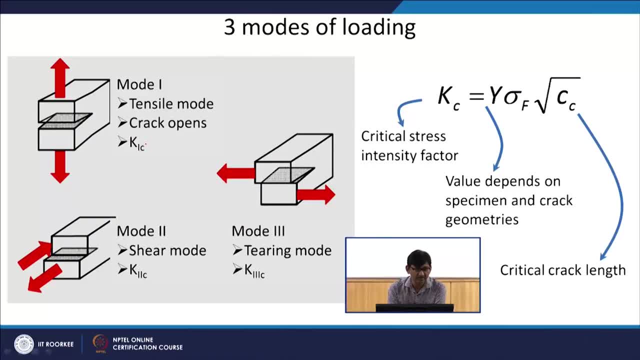 So when the mode 1 is there, then we critical intensity factor will critical intensity, stress intensity factor will be called as K1c. Okay, Because we are doing it in mode 1.. So which mode we are doing, that also we can include in the definition here. 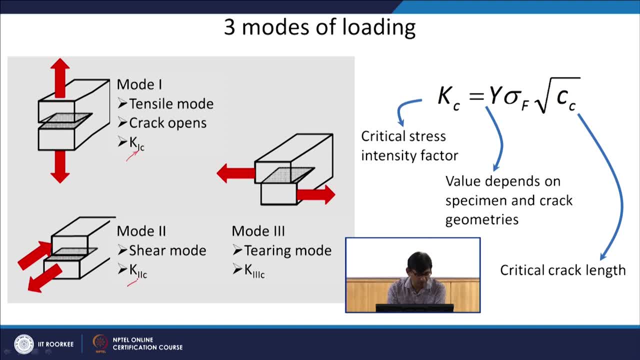 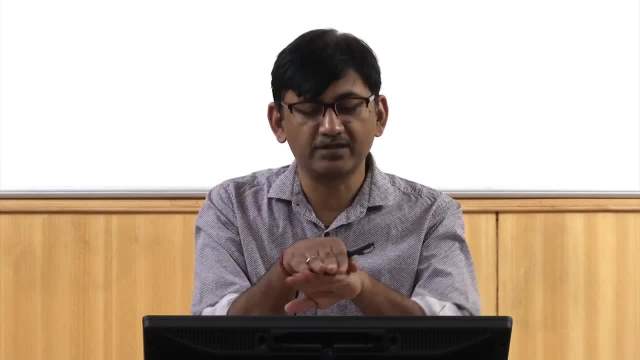 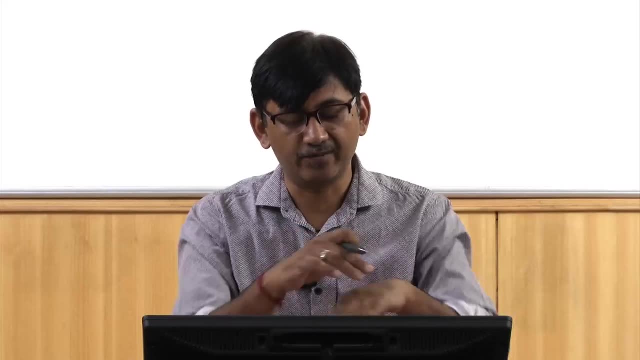 Similarly, mode second: when it is a shear mode, then it is a mode 2, okay, Then I will call it as K2c, And then if it is a tearing mode, so it is a mode like this, okay, So instead of shear mode like this, it is a kind of tearing mode, okay, and then it will. 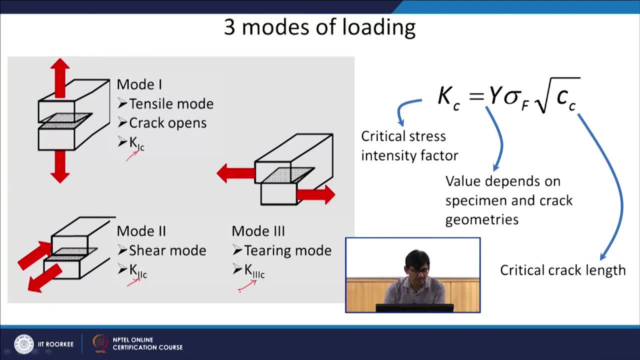 be mode 3.. So K3c will be written. Usually most important is K1c, which we will use in all the design practices. okay, So if you want to consider this geometry of the loading and geometry of the specimen, okay. 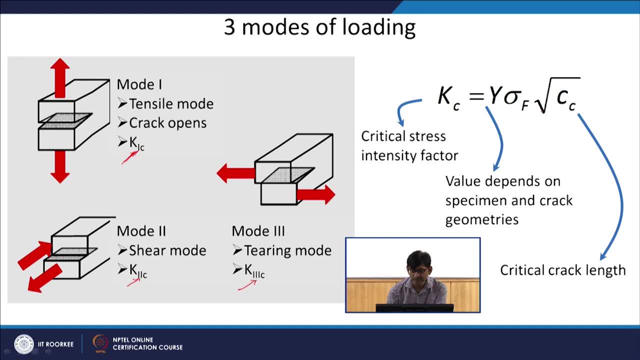 Actually, I can modify the equation here now. okay, So it will be critical. stress intensity factor: okay, Equal to a factor which deals with the shear- Okay, Okay, Equal to the value. depends on specimen and crack geometries: okay, and this is your critical. 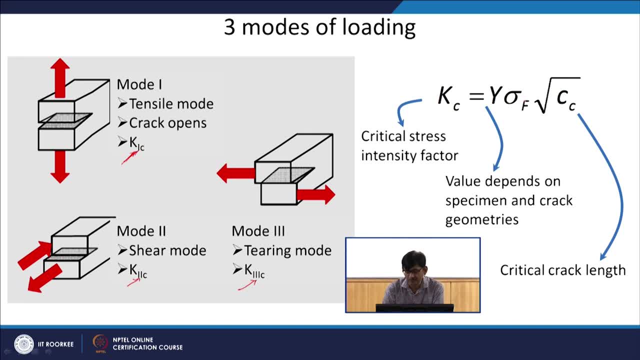 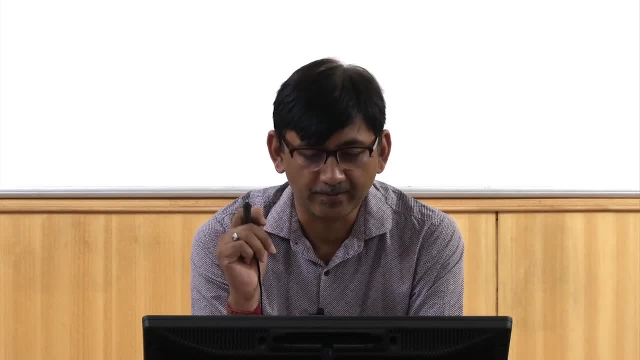 crack length and sigma F, your. as I told you, the fracture stress. okay, So stress at which the fracture takes place or the crack propagation becomes stable, If a very sharp crack can be made in a material. so now how we are going to use this particular 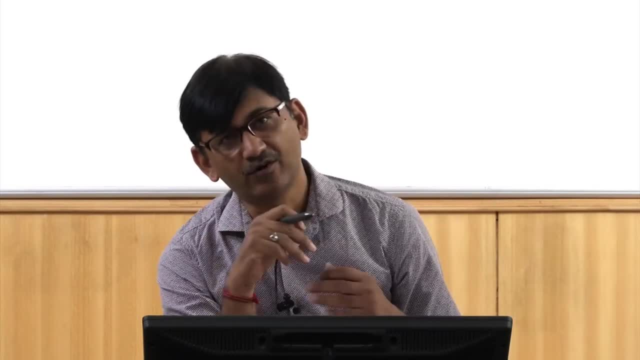 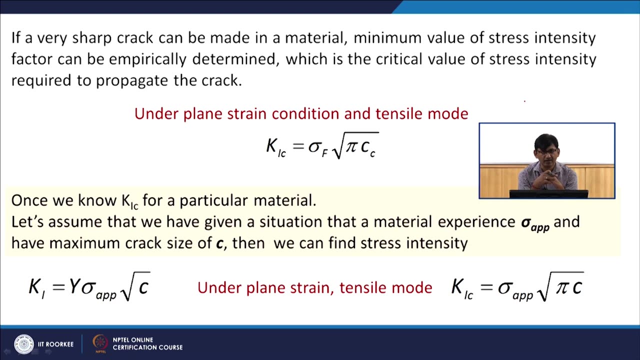 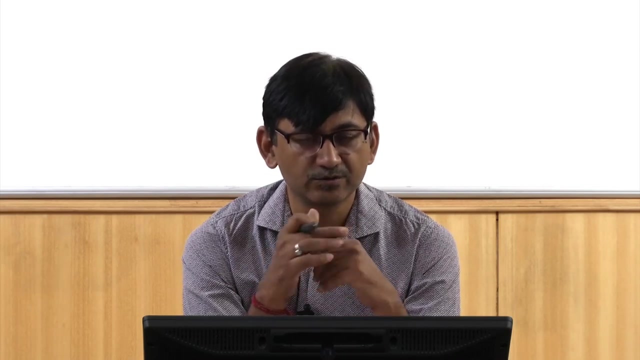 parameter, okay. So initially, what we will do is we will introduce a crack in the material, okay, So suppose we have a crack. So suppose you give a material to me, okay, and ask me to find out the that, what will be the critical intensity, stress intensity factor for this material? okay, 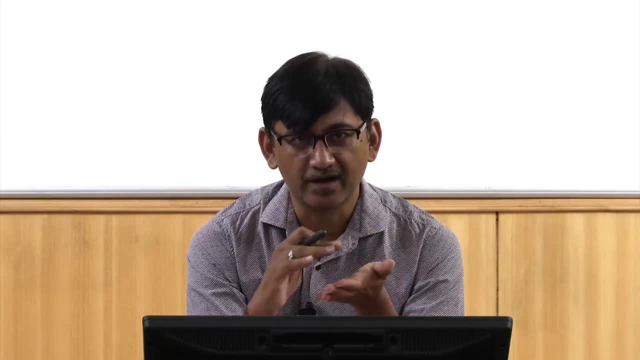 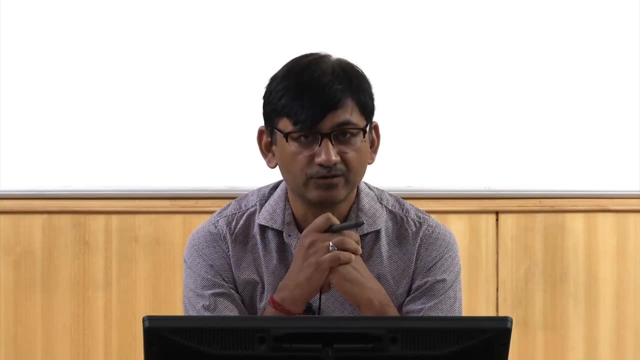 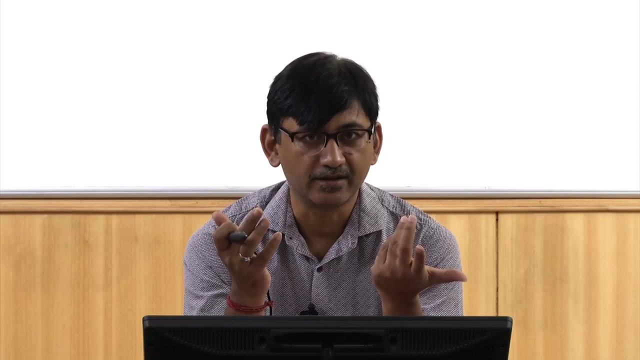 So what I will, we will do, is first we will make a specimen, introduce a crack of a known length which we have already introduced, okay, which we can easily measure, So that crack length we will always already introduce in the material, and then we will do test. 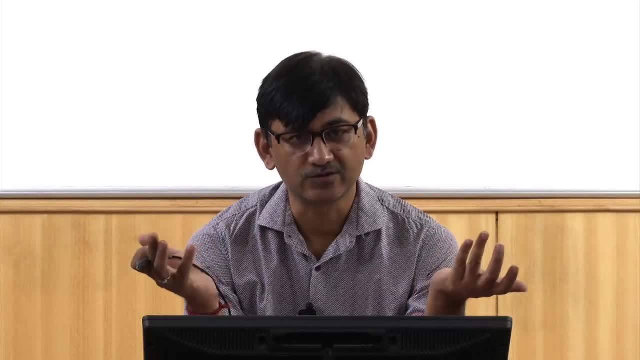 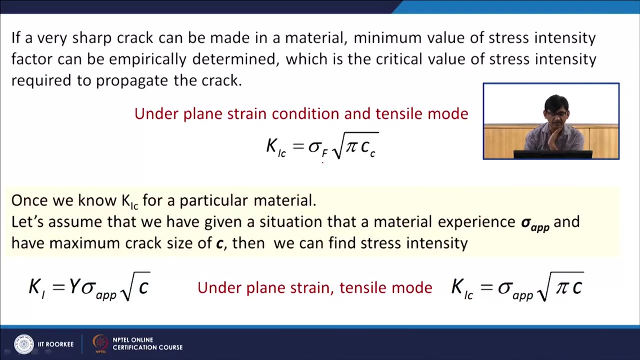 So to find out that at what stress it is going to fracture. okay, So when I do that, so under plane strain condition and tensile mode, which is K1c, I will find out that for a particular crack length, what is your going to be the fracture stress? okay, 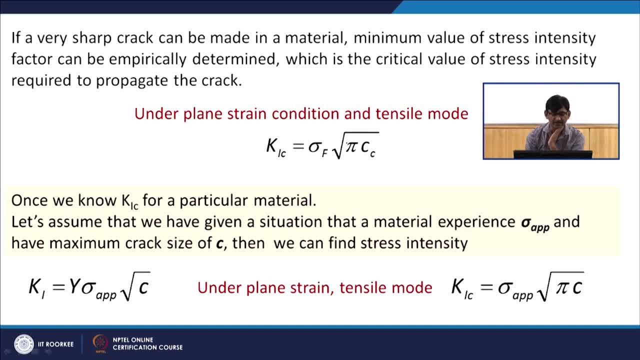 So by doing this kind of experiment empirically, I can determine that what will be the critical value of stress intensity factor? okay, So for a given material? Okay, So I get that Now. once I get that, now I am using this material in practice. okay. 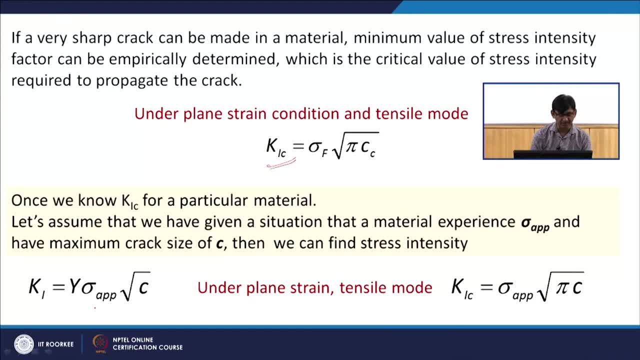 So there is in that practice, wherever I am applying this material, there will be some applied stress. okay, By doing some non-destructive testing, I can also find out that what are the typical crack or defect present in that material? okay, So by knowing this applied stress which you have found out from your design, okay, 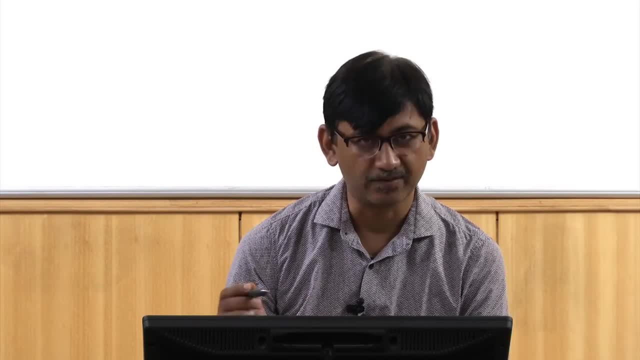 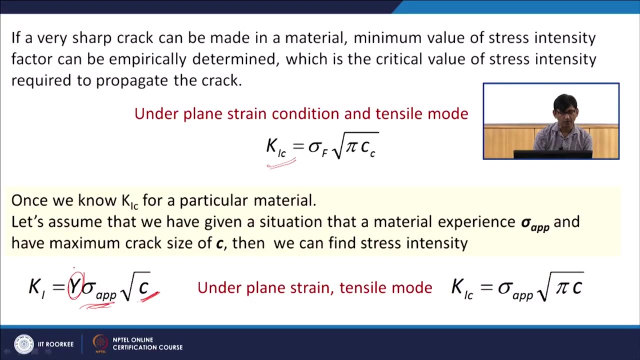 And finding out this crack length from some entity, kind of analysis, evaluation, okay, And using whatever geometries we are using, if we are doing it in plane strain condition under tensile mode, then Y will be under root pi. okay, I can calculate that. what will be the stress intensity factor under mode 1, okay, 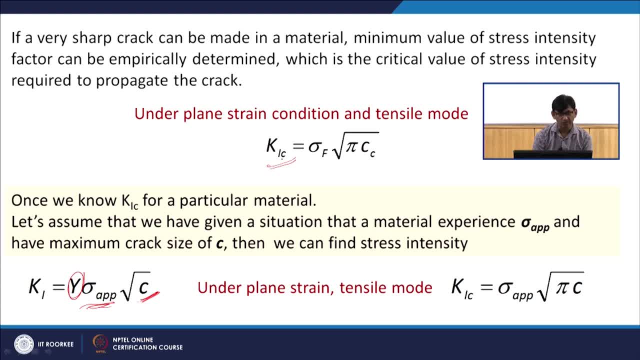 Now, if this is stress intensity factor is more than K1c, Then I can calculate that what will be the stress intensity factor under mode 1, okay. Now, if this stress intensity factor is more than K1c, Okay, Then I have to either change the applied stress or I have to redesign the my structure, or 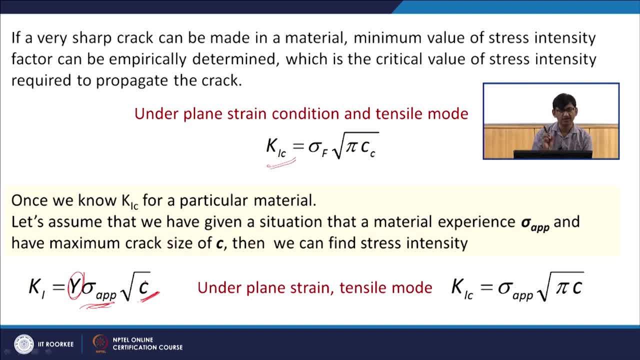 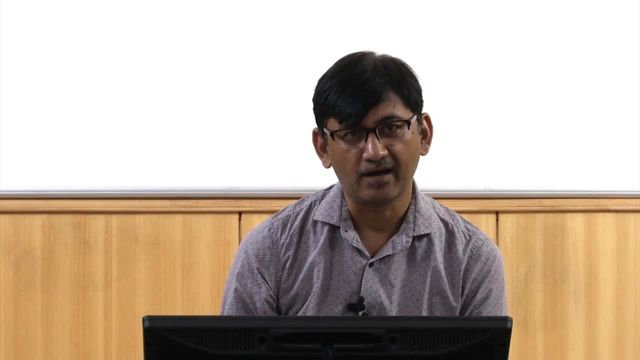 I have to do certain processing to the material to reduce the defect size. So if K1 is more than K1c, If K1 is less than K1c for this given applied stress and the whatever defects are there in the material, Then I can say that this is a safe mode. 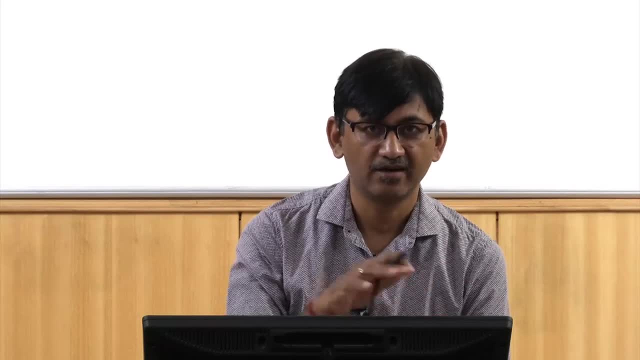 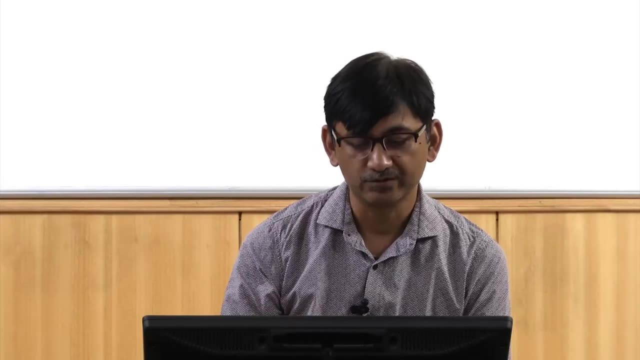 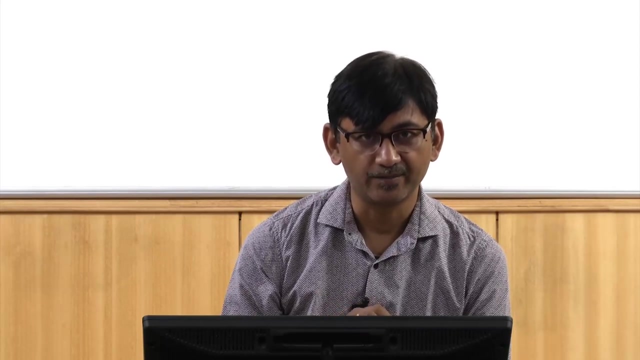 And I can use this material under this stress condition with the given flaw size. okay, So I guess you understood that how we are going to use this stress intensity factor to find out the whether I am going to or whether I will be able to use a certain material with. 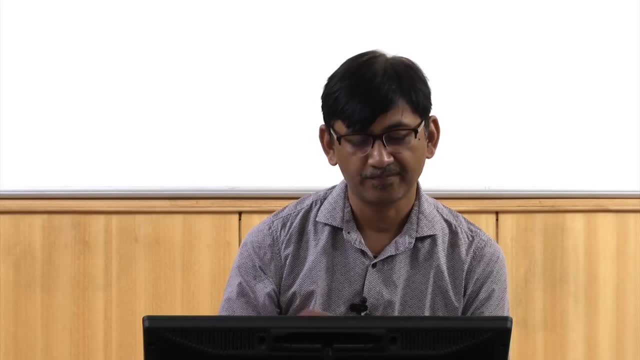 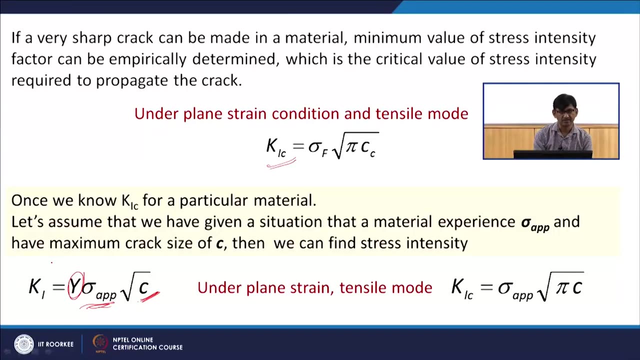 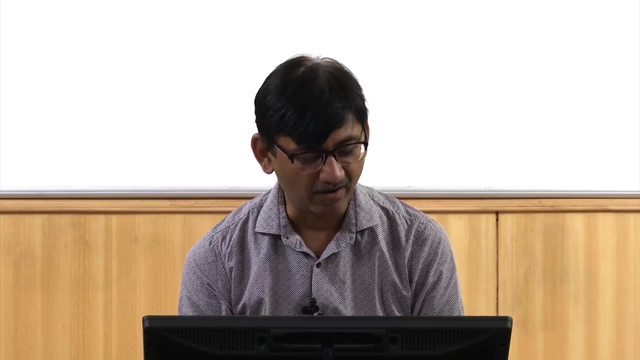 certain crack length under certain applied stress. okay, And by comparing the critical stress intensity factor with the stress intensity factor. Okay, Thank you. So the stress intensity factor we have calculated for a particular condition. okay, So in books I have found that there is lot of confusion regarding these equations. okay, 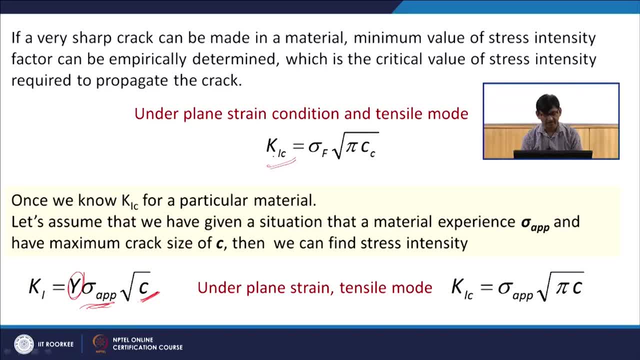 I have done. whatever I have followed here is that K1- the 1, is your tensile mode and in plane strain condition, and C is your critical when we are talking about critical. So when we are talking about critical, this stress should be the fracture stress. 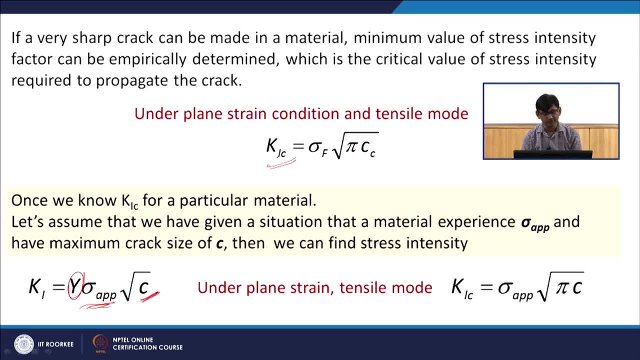 Okay, So under root pi term comes only when I am using K1, okay, As you can see, here also I am using K1, okay. So let us say I am not going to use K1 here. okay, And I will be using only K, So Y. when I put Y as under root pi, then I will use it as K1,. 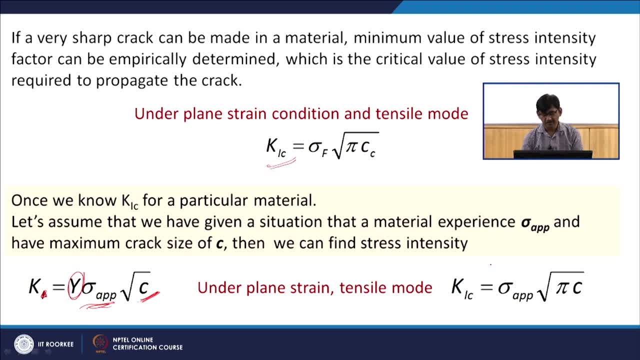 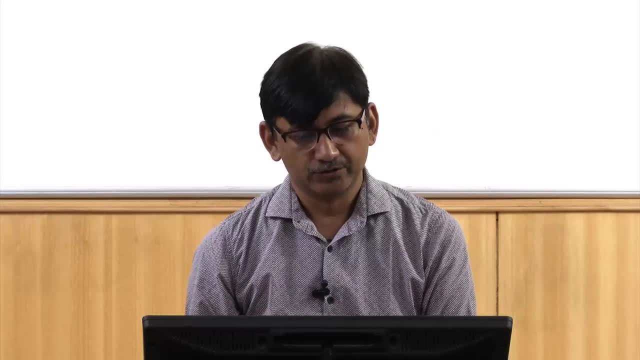 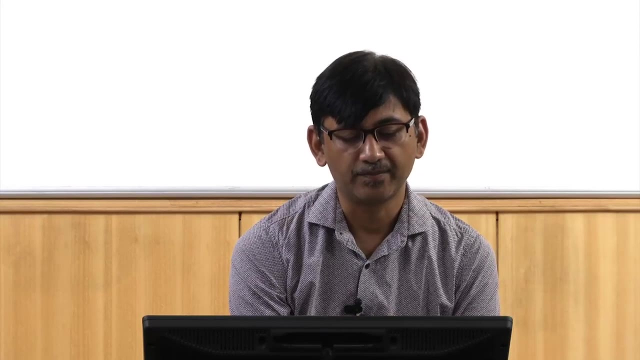 okay, So under plane strain tensile mode: okay, this is what I will get And I can compare with the stress intensity factor which I am calculating and find out whether I can use this for a particular application or not. So, as I told you that in general, I will write. it. is K equal to Y sigma applied under root. 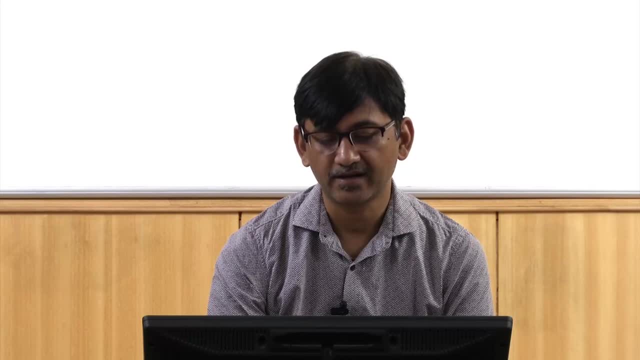 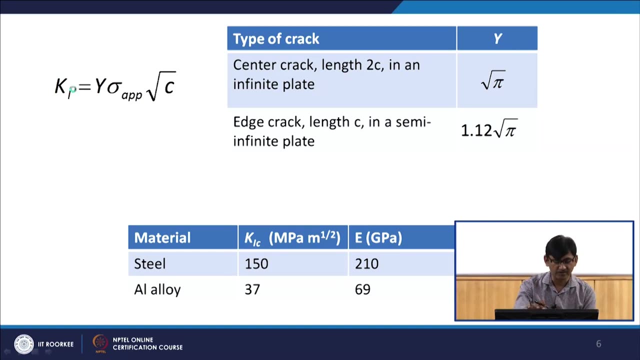 C, Okay. So if it is a crack length centre crack with length 2C in an infinite place, Okay, Okay. So under plane strain condition. So one I can always use because one is for plane strain. sorry tearing mode, sorry tensile. 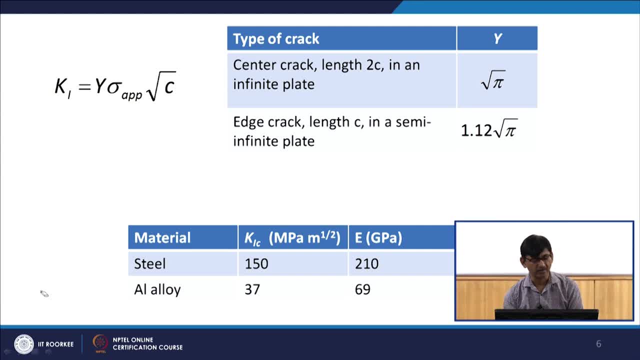 mode. Okay, So one is for tensile mode, So I can use that. and why? I will put only according to what kind of crack is there. So if it is a centre crack within the material, through crack with length 2C in an infinite. 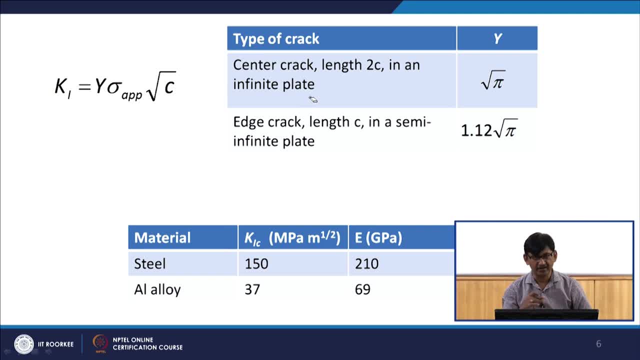 plate. So it is a plane strain condition. for infinite plane, The condition for deformation will be plane strain. For another set of conditions, Y will change. Okay, So it is a edge crack. So then I will use a factor like this: Okay. 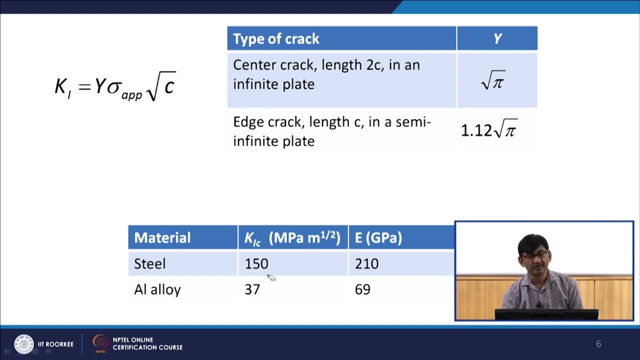 And then there are some values for the critical stress intensity factor For steel it is around 150 mega Pascal per meter under root meter actually. Okay, Okay, Okay. Now it is under root meter and aluminium alloy it is around 37. Okay. 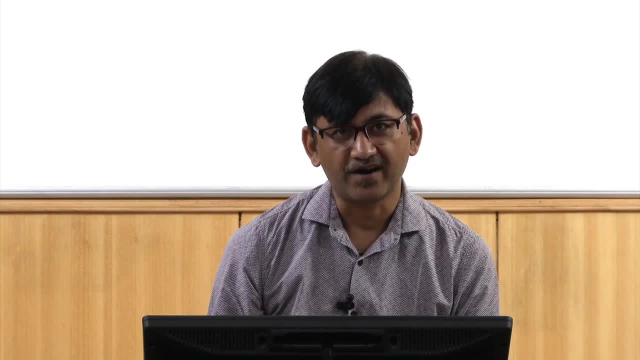 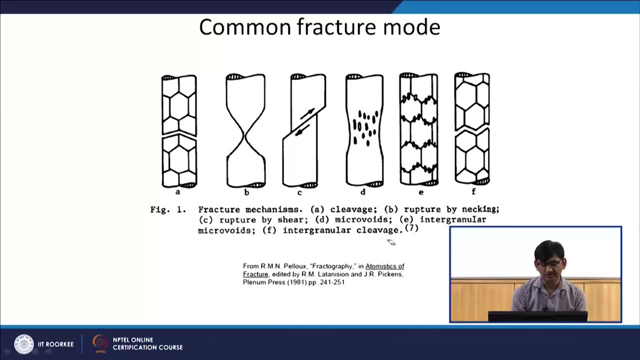 And their Young's modulus is also given here. Now, what are the common fracture modes? Okay, So if you see the there are different fracture modes already we have seen once in the previous slide also. Okay, Just to recap here. So in this case the crack is going through the grain. 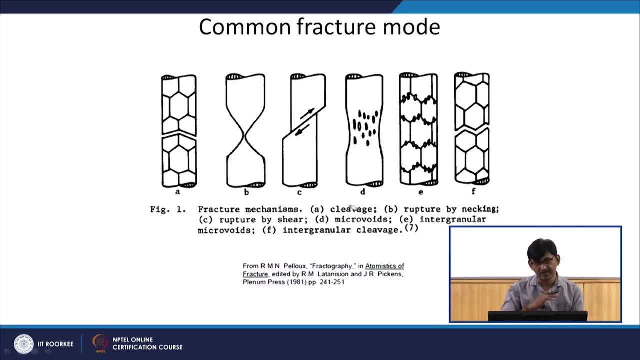 Okay, And this is what we call as cleavage fracture, through the, through the crystallographic plane. Basically, the crack goes through the crystallographic planes. So, as you can see, a certain plane is preferred, So it is going through that in that plane may be oriented in a different way in next. 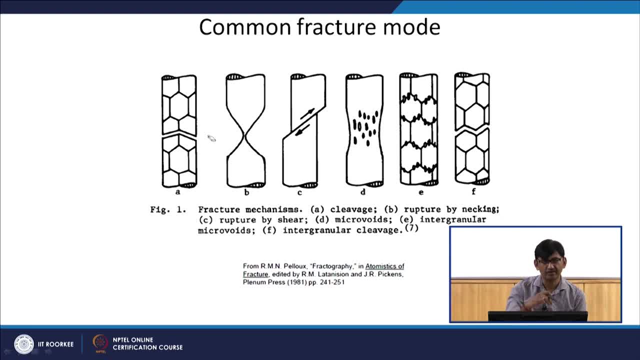 grain. So the crack has kind of there is a divergence or diversion of the crack in that next grain, But the crack will go through the grain, Okay, So in this case the it is a transgranular fracture. The another fracture, which is a ductile fracture, can be there through necking process. 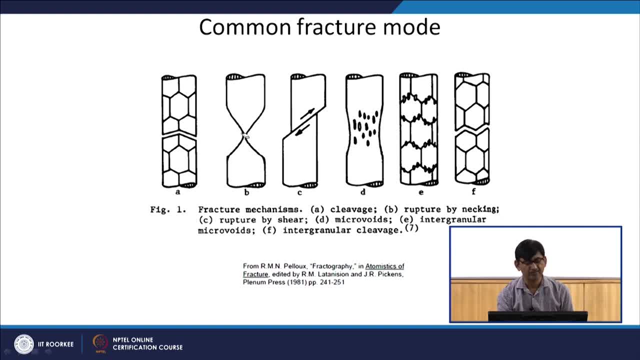 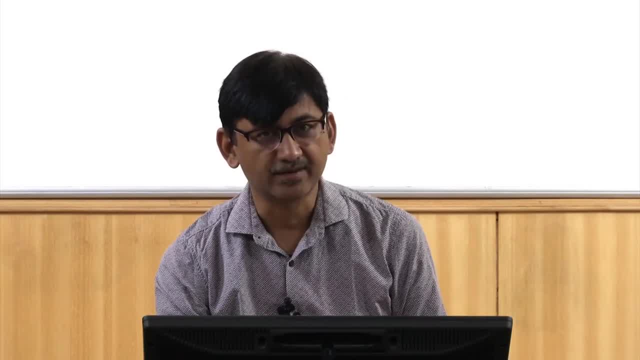 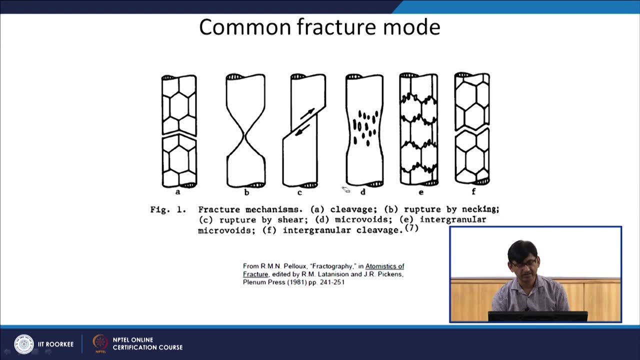 So it is necking, Okay, And later on it will fracture, when the diameter of the material become very small. Then this is the rupture by shear process. Okay, Under plastic deformation again, Then there is a micro wide coalescence. we will see this when we will discuss the ductile. 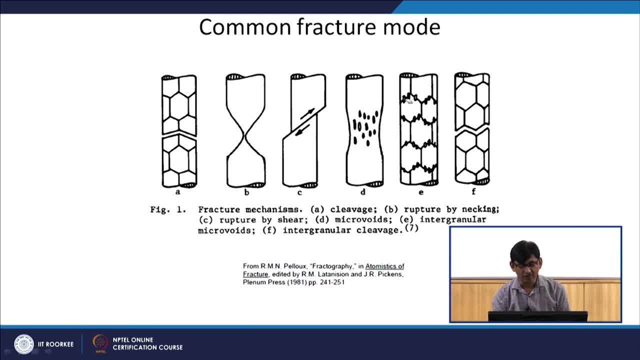 fracture, Okay. Then there can be voids on the grain boundary. Okay, So then it is intergranular micro voids or intergranular cleavage. So in this case now the crack is going through the grain boundary. In this case the crack was going through the grains. 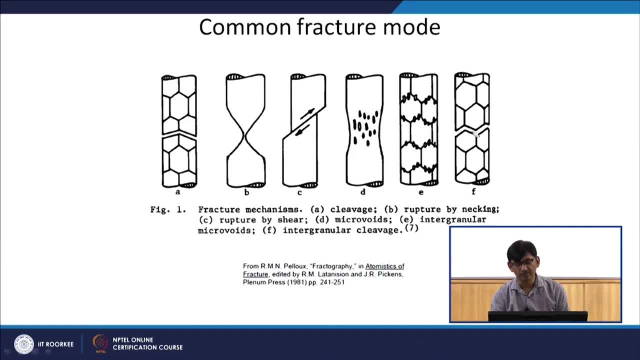 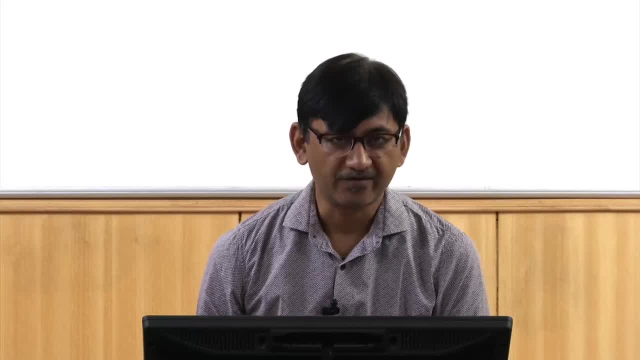 So crack can also go, can go through the grain boundary. Okay, Then it will be intergranular cleavage. So now we will look at different type of fractures. So first is brittle transgranular fracture. So first is brittle transgranular fracture. 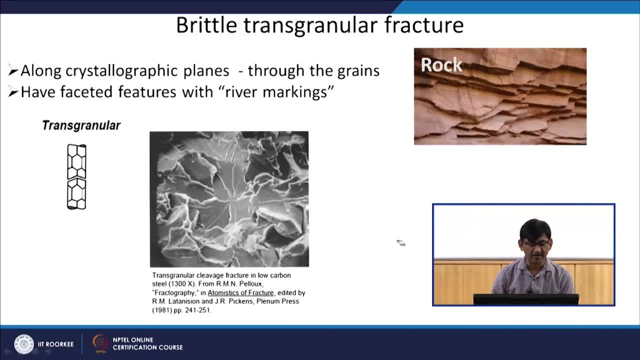 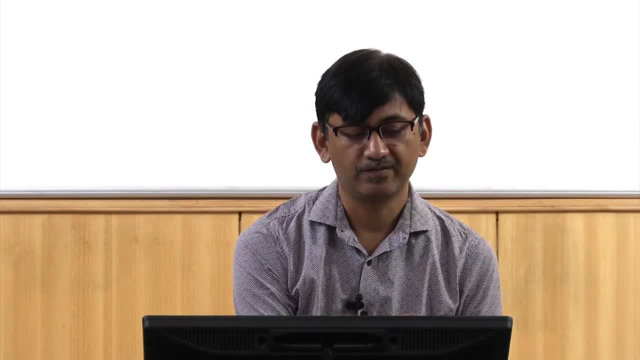 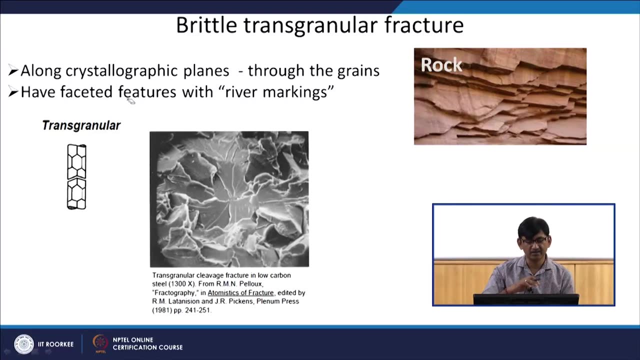 So this is the crack, This is the fracture. Okay, That means through the grain. So when you have a brittle transgranular fracture, Okay, The crack is propagating along the crystallographic planes or through the grains and usually it gets you get a faceted feature with river markings. 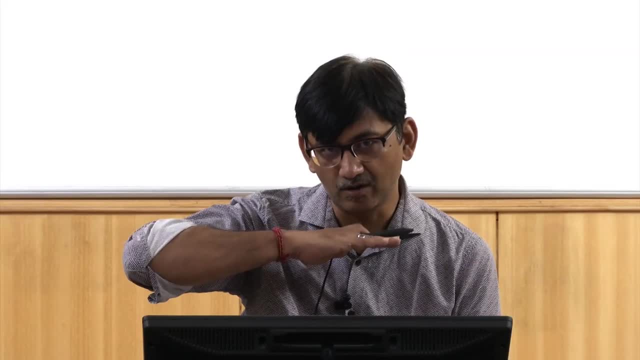 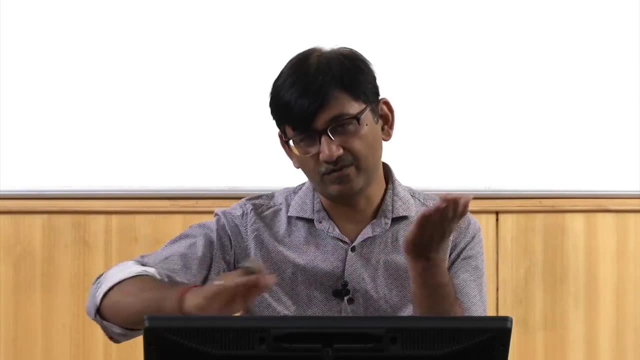 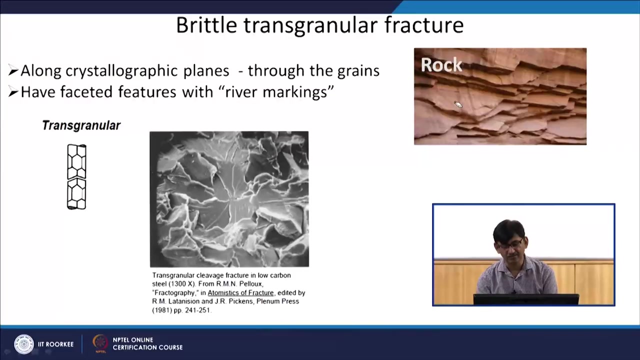 Faceted feature because the crack is going along a certain plane, So you get one facet in another grain. Okay, It is oriented in a different way, So you get another facet, and so on, And usually at macro scale you can see this kind of fracture very nicely on a some rock. 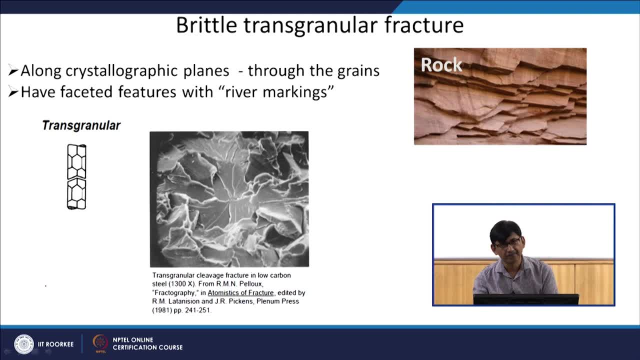 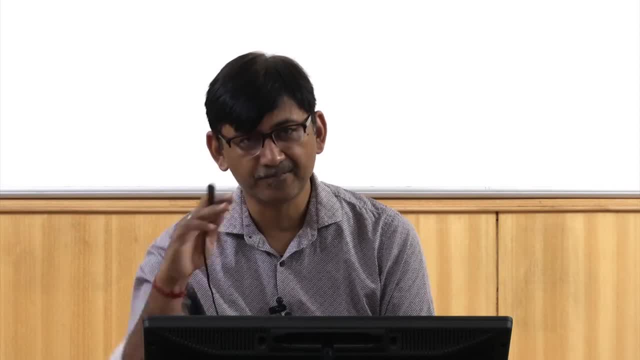 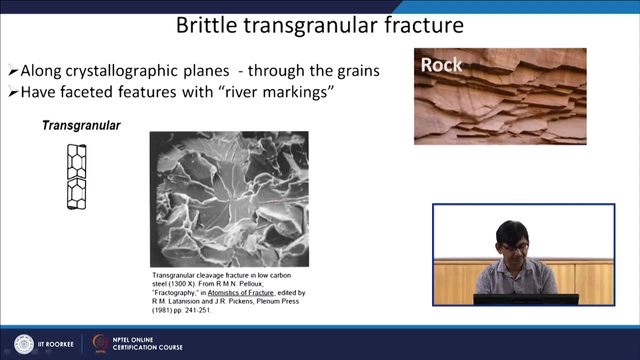 if some fracture is taking place or there is some crushing of the rock is taking place. as you can see very nicely, these kind of facets are there on the rock sample at a macro scale. Okay, This is a scanning electron micrograph of fracture sample. 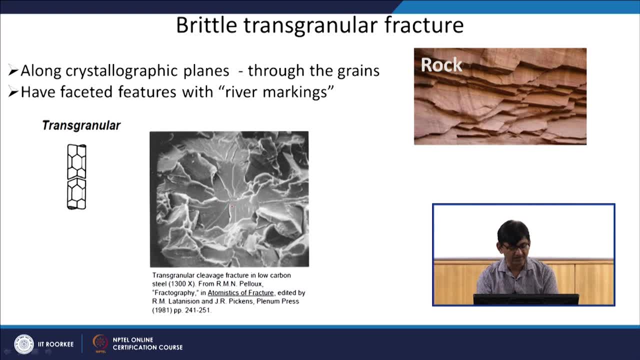 Again you can see the facets. So one facet, one facet, and when, wherever the grain boundary may be or wherever the crack is going into another plane, Okay, You get this kind of river marking, So it kind of where the crack has changed it path. 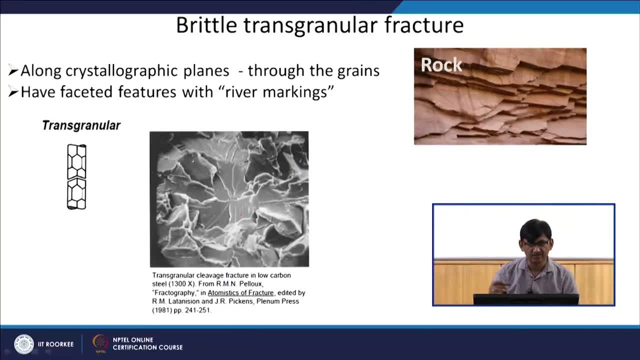 Okay, You see this kind of river markings. Okay, So it is like tributaries to a main river, that is how they come, and then they join the main river. Okay, So that is why it is called river marking. Then a brittle fracture gain also happened inter granular. 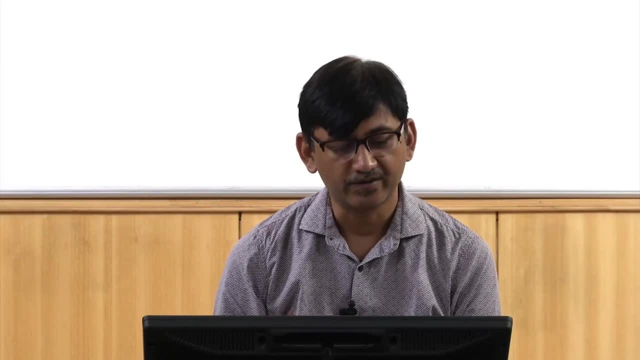 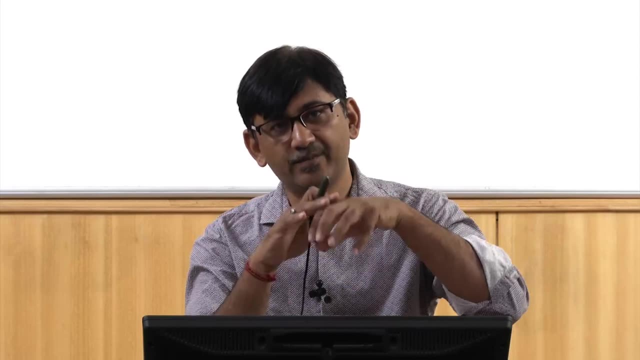 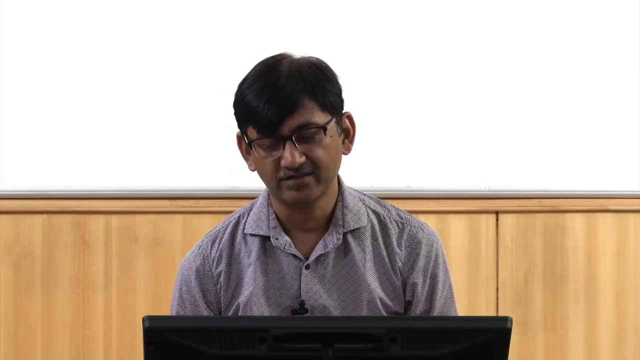 Okay. That means the crack will propagate through the grain boundary. So in this case you get a granular appearance. Okay, Because it is going through the grain boundary. So the shape of the grain is actually Okay, What you see very nicely on the fracture surface. 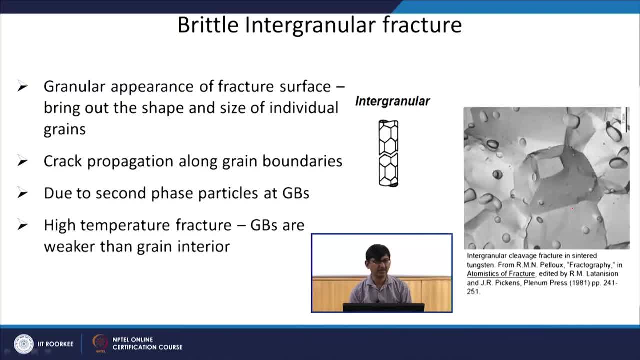 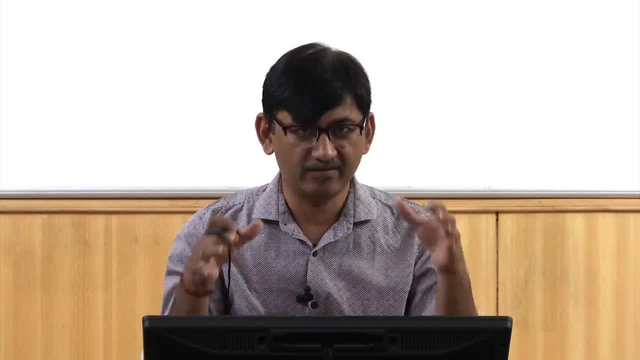 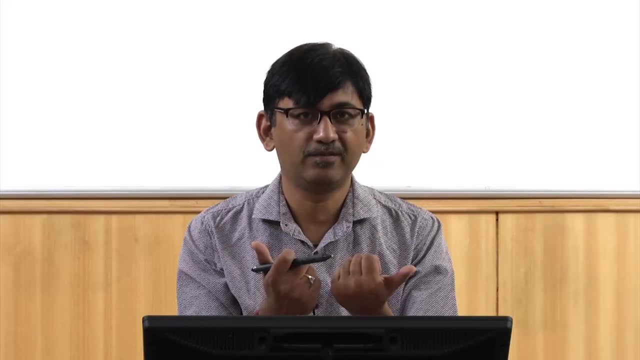 If you want to compare this kind of fracture with anything which you see in a day to day life. you take a thermocol- Okay, Those white packing material in which you get all these electronic equipments, your monitor and so on- and you just fracture that thermocol. 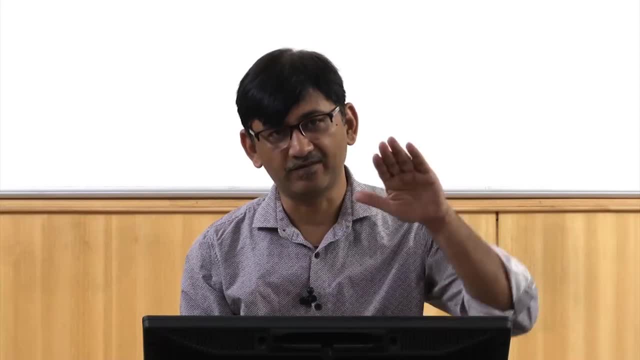 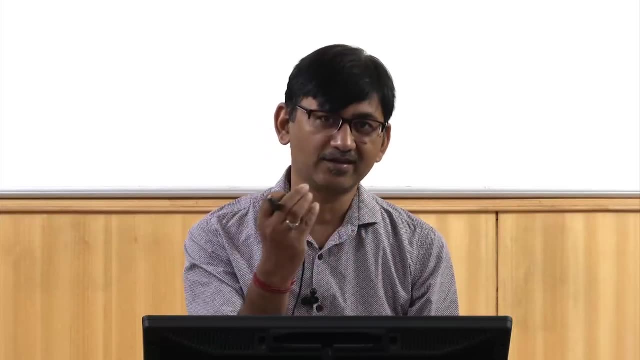 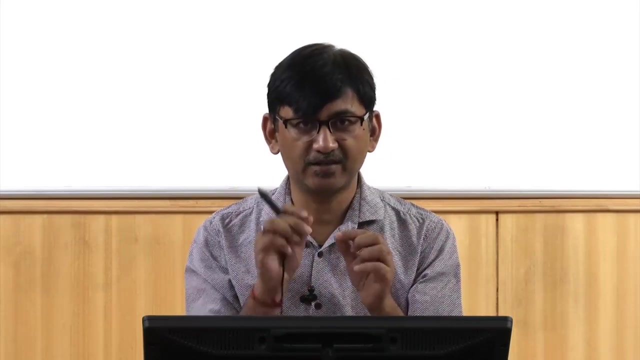 Okay, Just break that thermocol, Okay, And whatever the surface, you will see. that is how you will see a inter granular fracture, So those individual thermocol grains. that is what you will see and in that the fracture is actually taking place between the two balls of thermocol. 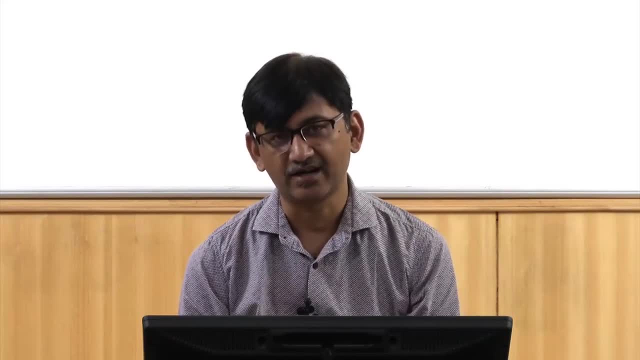 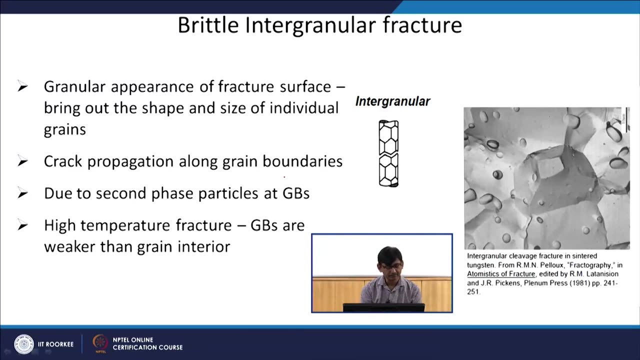 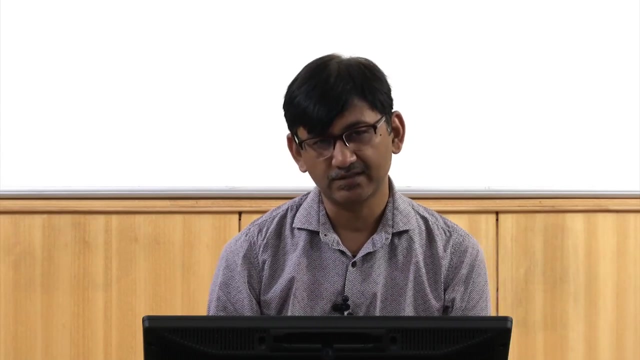 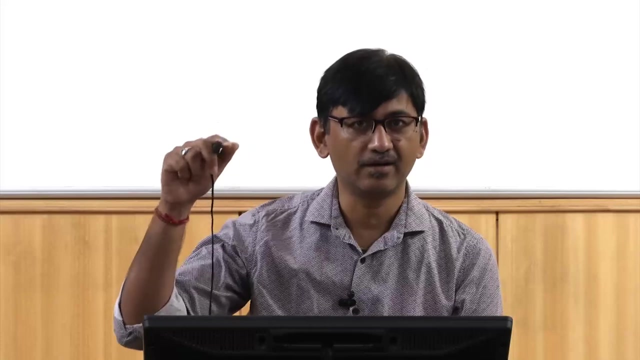 Okay, And that is what you will see very nicely, this kind of fracture feature. So in this case the crack propagate along the grain boundaries. Okay, You, And why it takes place. suppose you, if you remember, we discussed, when we were discussing about steels, that in hyper eutectoid steels the cementite form on the prior austenite 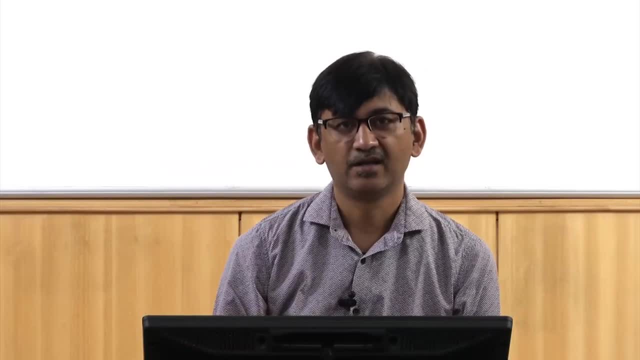 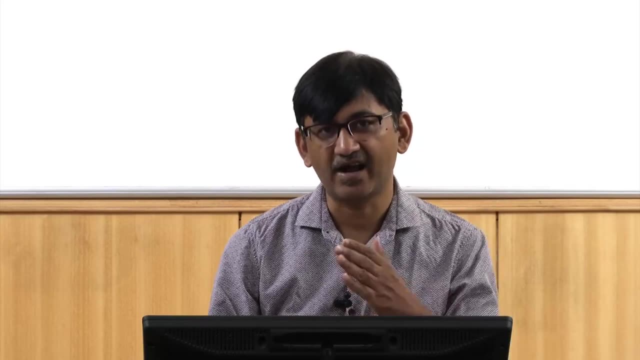 grain boundary. So it is kind of a continuous network. So if you have this kind of microstructure, the cementite is a brittle phase Okay, And if any crack nucleates it is very easy to propagate the crack through this cementite network. 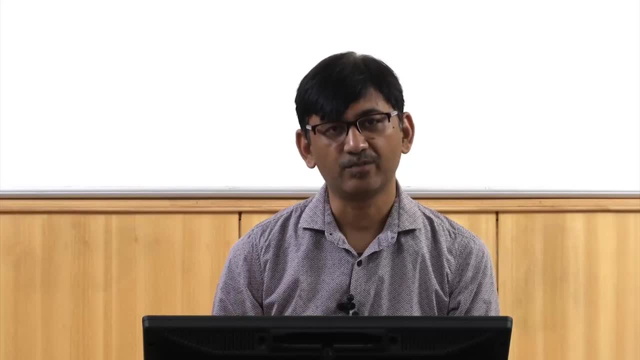 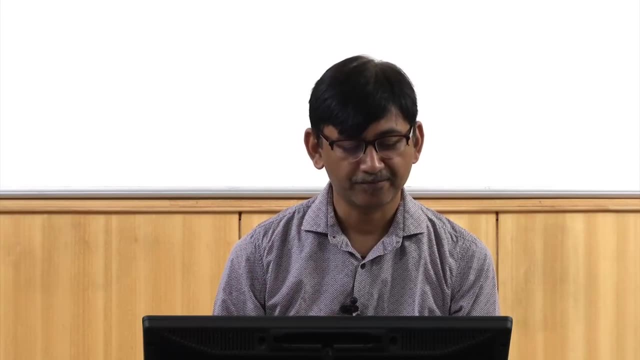 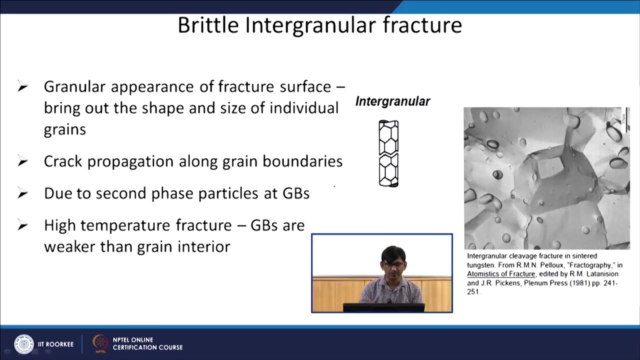 Okay, And because this cementite network is on prior austenite grain boundaries, you will see a nice granular type of fracture features. Okay, So this: if you have on grain boundary a continuous network of second phase, then the crack will propagate, may sometime can propagate through grain boundary. 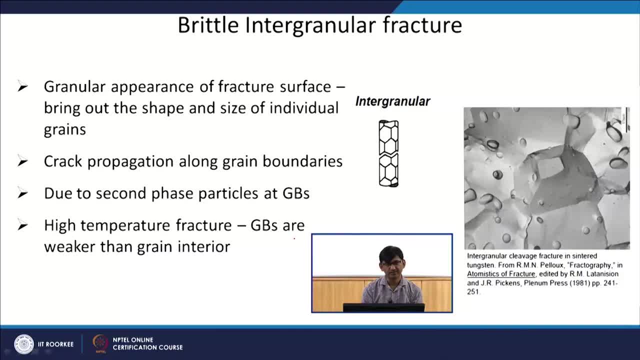 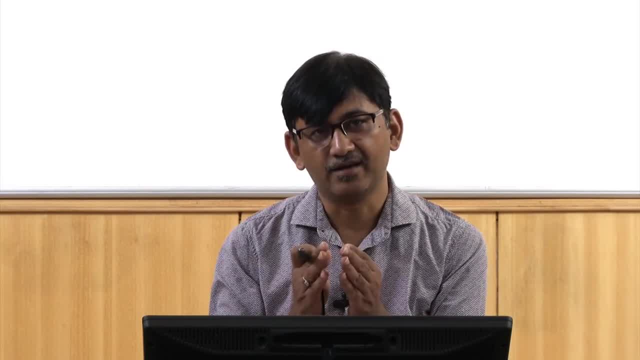 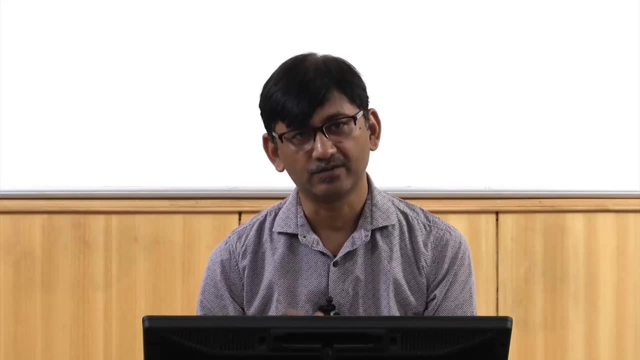 In high temperature also. this grain boundary fracture takes place because at high temperature, grain boundary is weaker than the grain. Okay, They are already quite easy to separate at high temperature, Okay, So the crack propagates through the grain boundary when you have high temperature fracture. 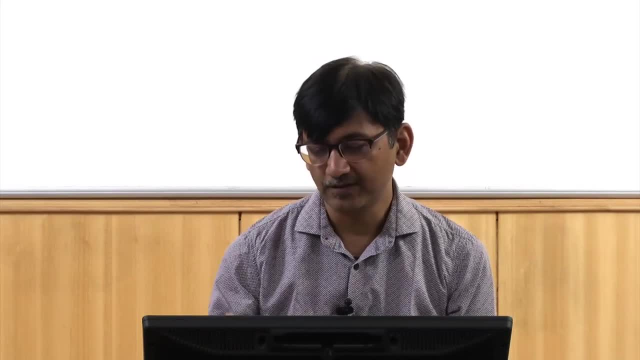 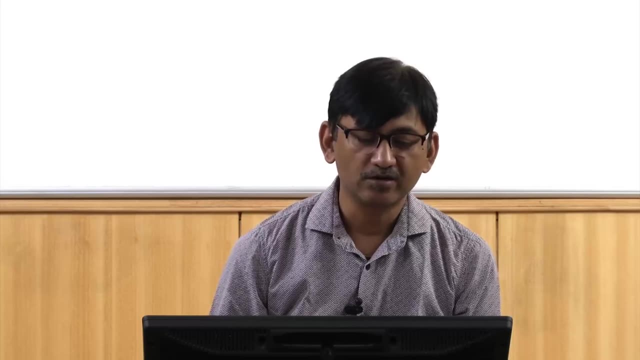 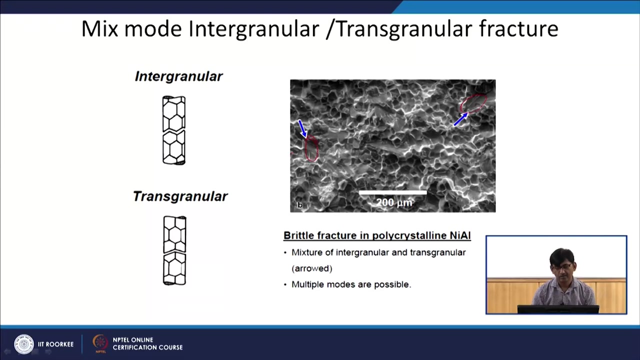 Okay, In some cases- not always So- in high temperature fracture also. you will see this kind of fracture feature Sometime. it can be mix mode also. you can get inter granular, you can get trans granular. Okay, You can see, these are all with faceted features. 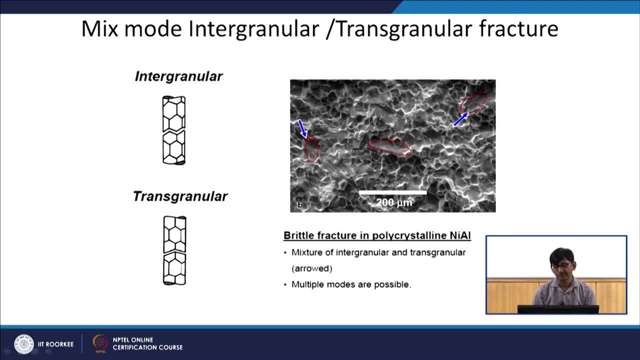 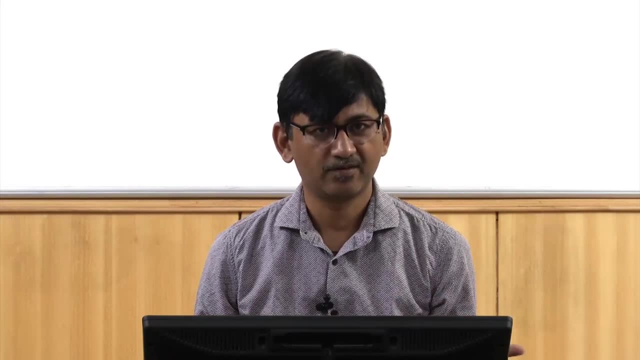 Okay, You can see a faceted feature here also. Okay, So there can be sometime mixing of two different fracture modes, also because in practice things are not very simple. Okay, You have very complex stress system. Okay, Material is experiencing different stress state at different places, so the fracture 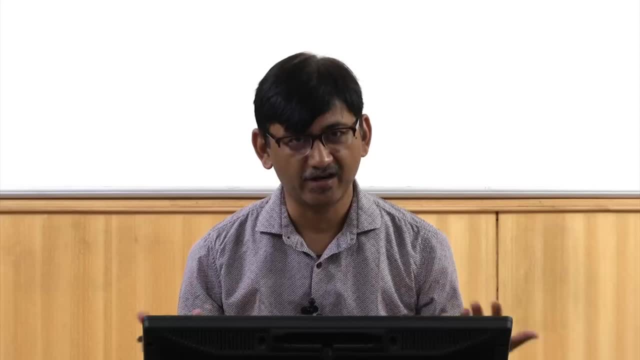 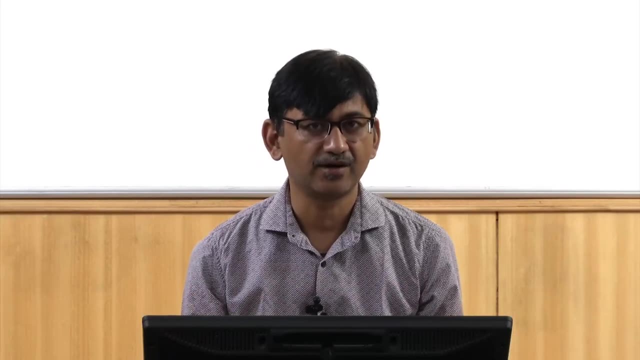 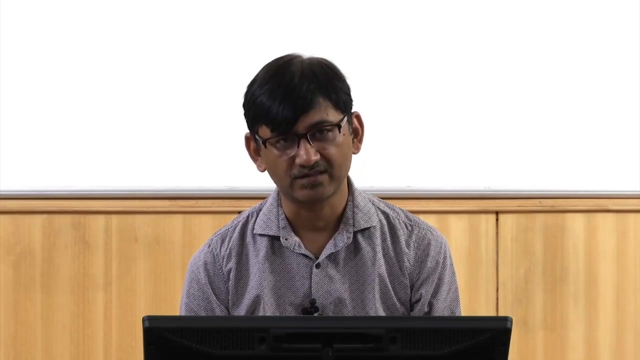 can also be of different type. Okay, And if there are two multiphase material, some phase will deform by, or crack by, trans granular mechanism. another phase may fracture by inter granular mechanism. So you can get a mix mode type of fracture features on the surface. 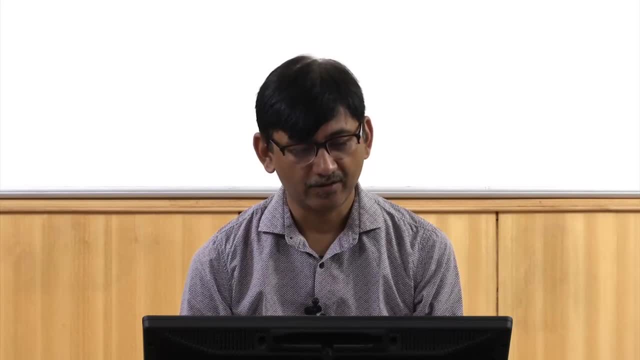 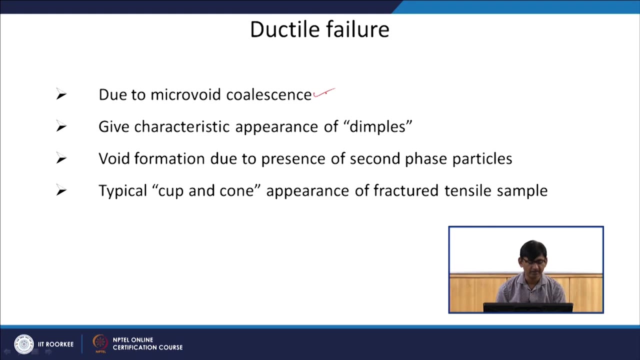 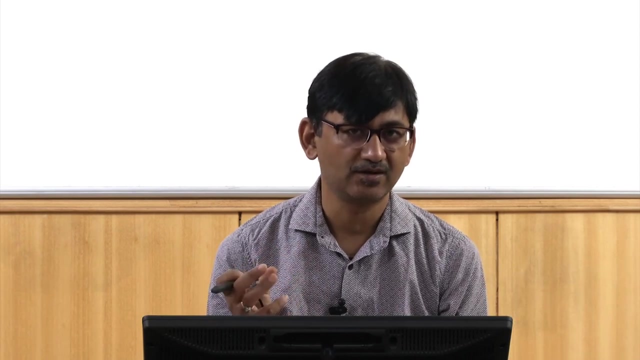 Now coming to the ductile failure. Okay, Or ductile fracture. This is: this happens due to micro void coalescence, So we will see. what do we mean by that? Give characteristic appearance of dimples. Actually, this is what we call. what features which we see on the for ductile fracture? 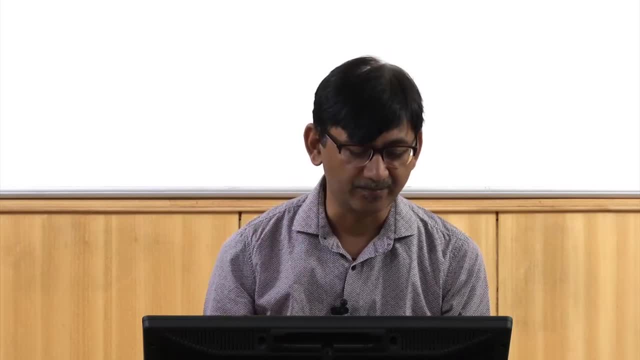 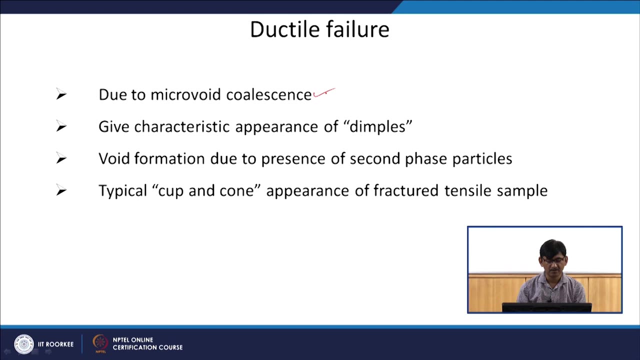 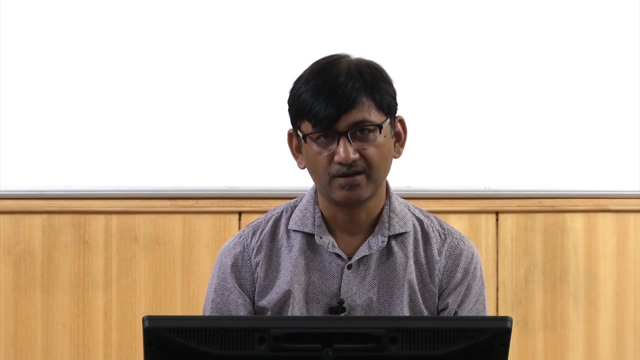 Okay, We say that these are dimples. Okay, It looks like dimples. Void formation due to presence of second phase particles. Okay, And typical cup and cone appearance of fractured tensile sample. So this we have already earlier also discussed that you get this kind of cup and cone type. 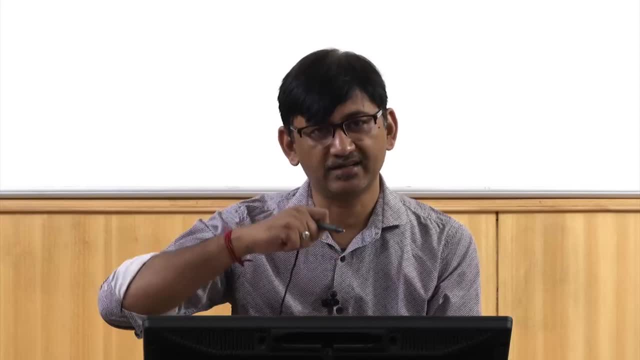 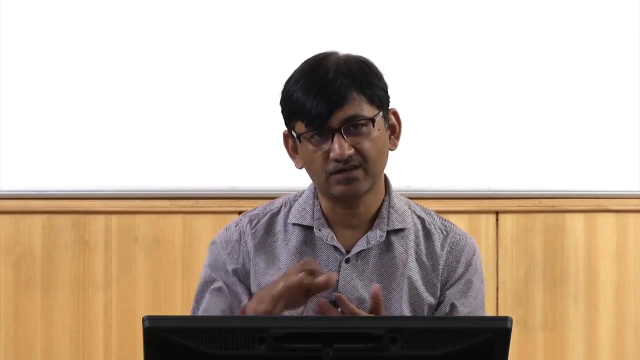 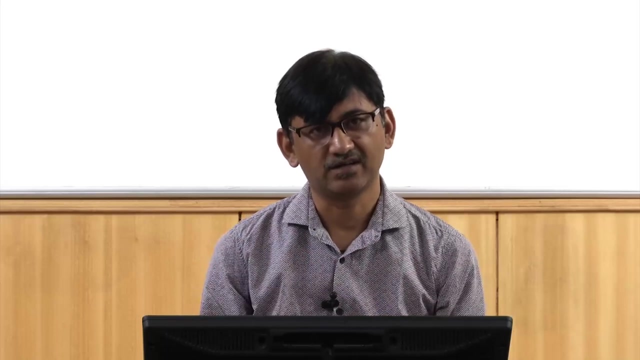 of fracture. So if you have a ductile material and you do the tensile test you get this cup and cone fracture appearance, Whereas if it is a brittle fracture you will have separation of two of the sample in two parts and almost fracture. macro features of the fracture: surface is flat. 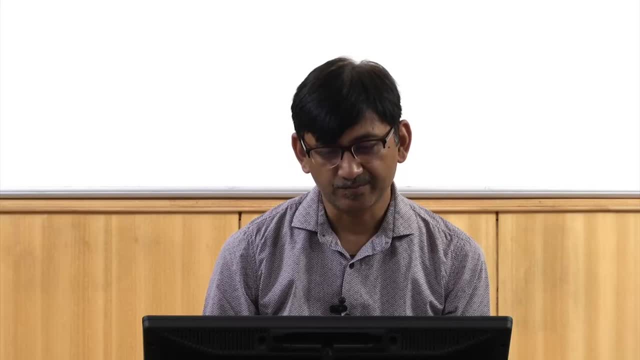 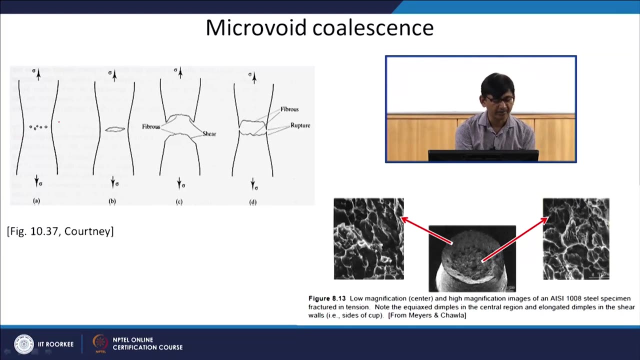 Okay, So what does what happens in this micro void? coalescence, Okay, When you are deforming and suppose necking starts at some point. Okay, Now there will be some this kind of micro voids which will be forming on the inside the 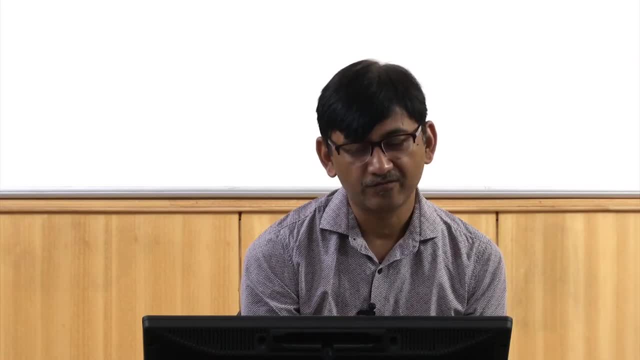 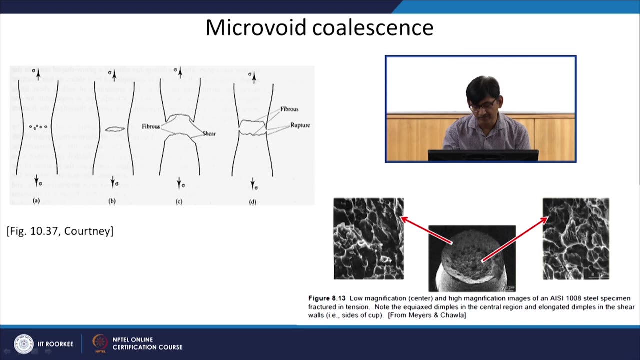 sample. Okay, Why this micro void form? Okay, Suppose you have some inclusion in the material, let us say inclusion or precipitate or whatever. Okay, And you are deforming. Now the mechanical properties of the precipitate will be different, Different than the matrix. 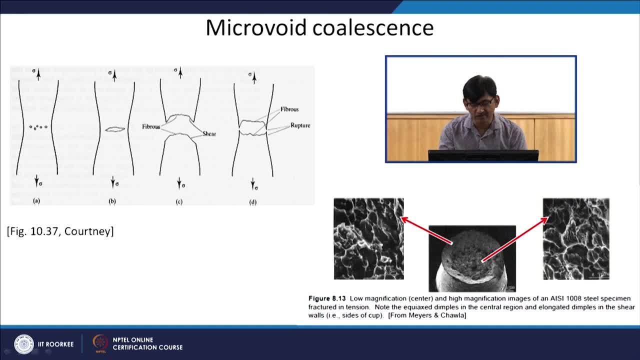 Okay, Usually precipitates are all very hard compared to the matrix. So matrix is soft, it can deform, whereas the precipitate will not deform. Okay, So when you have suppose this is my precipitate, this is my matrix around it, My matrix is able to deform, but precipitate is not deforming and there is an interface. 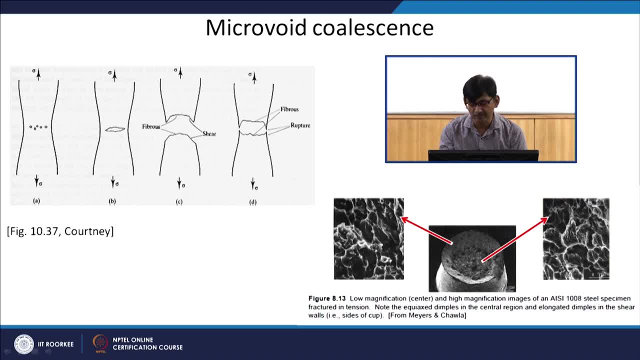 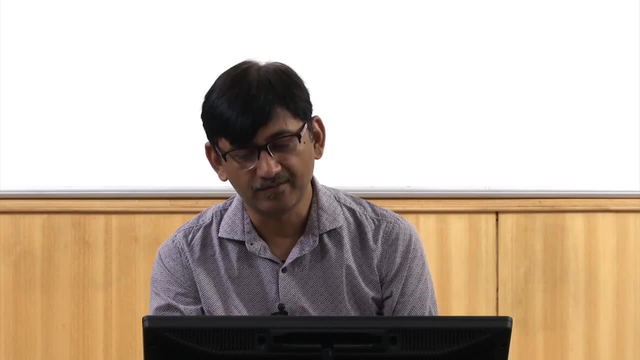 here, Isn't it? So what will happen? When it is able to deform, it will try to separate from the. my matrix will try to separate from the precipitate because it is able to deform, whereas precipitate is not deforming. It is kind of a solid, inflexible precipitate within the grain. 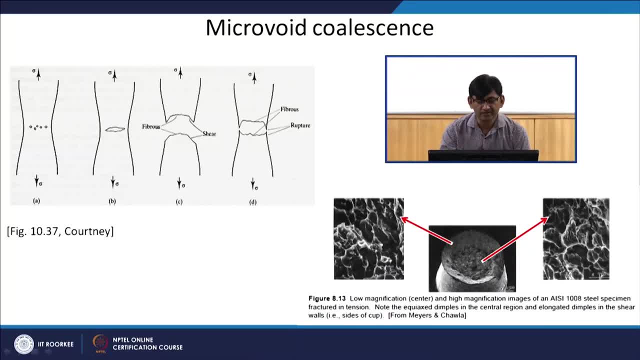 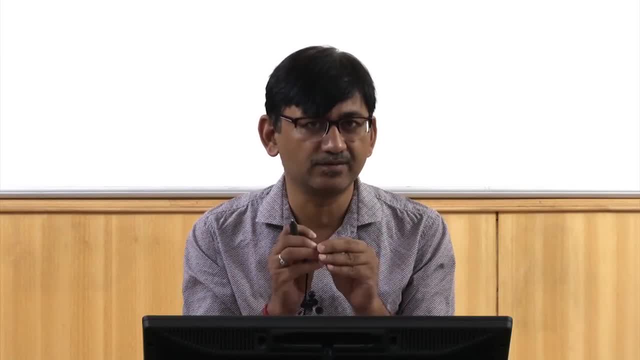 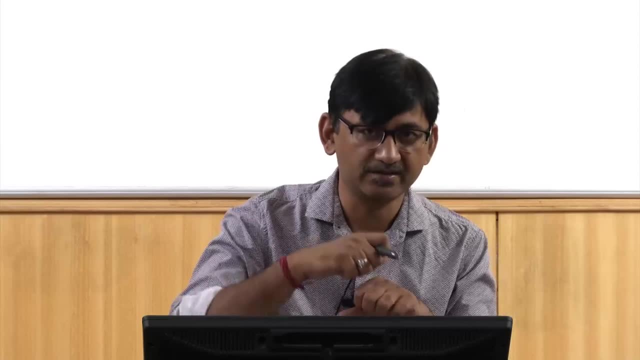 So what will happen now? you have initiated voids at the interface, Okay, And these voids, Initially these voids will be very small, Micro size, small voids- Okay. And when you keep on increasing the stress because of the making, there will be the stress. 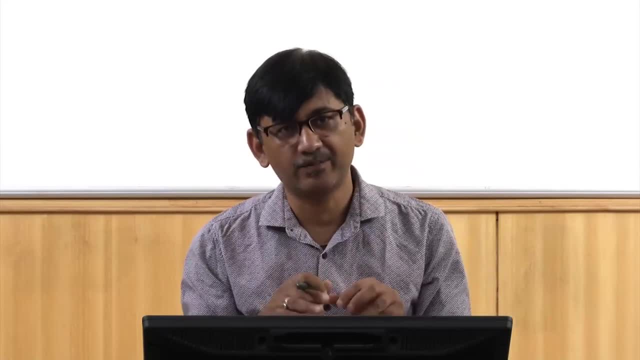 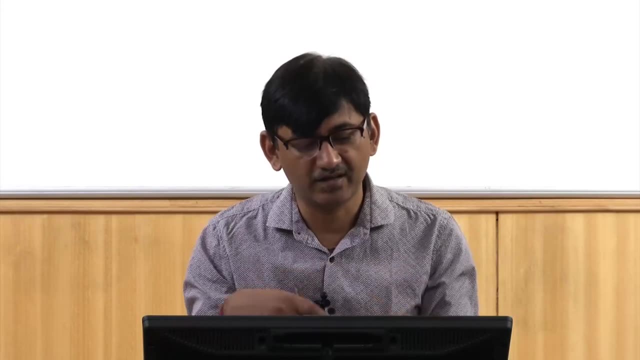 will be concentrating in this region. Okay, What will happen? that these voids will grow and they will start connecting with each other. Okay, That is what we call as coalescence. Okay, So first voids will form the small voids, micro voids. 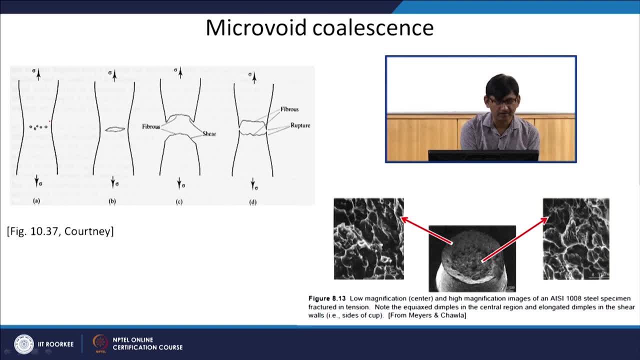 Then they will kind of connect with each other, Okay, And you will get a region within the material which is now already separated. So remaining material on the outside is remaining there, Okay, And that will fail in a shear mode. Okay, You can see that this is typical 45 degree shear surface. as I told you already that when 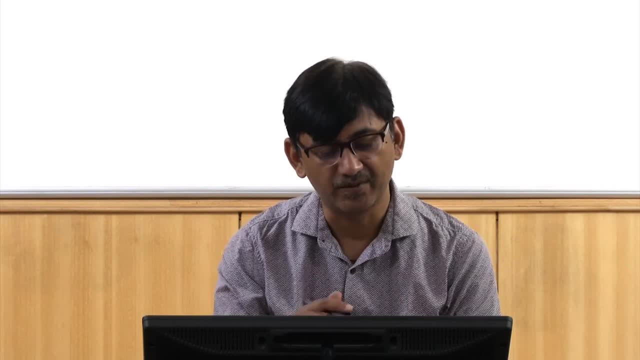 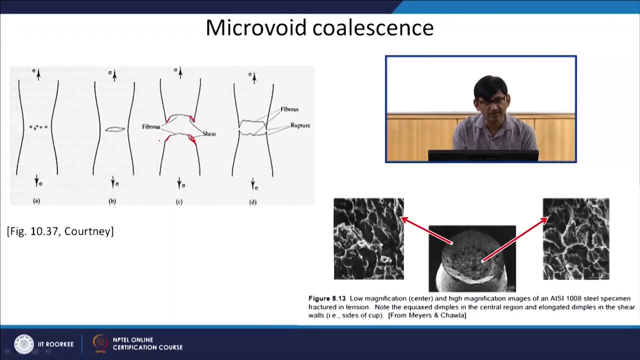 you have any axial tensile. at 45 degree you will get maximum shear- Okay. If the material is already separated from within, the remaining part will shear out- Okay, And at 45 degree almost Okay. So you will get a fibrous appearance here because of those micro void and they are coalescing. 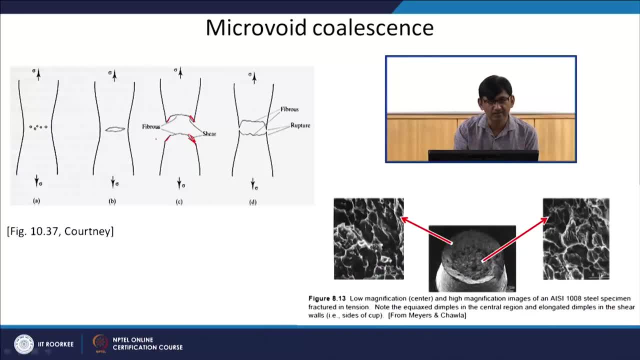 with each other and the shear on the outside, And this is what is going to give you a cup and cone type of fracture feature. Okay, You can see that there is a flat region and then there is a raised region here which looks like a cup, and in this case it looks like a cone. 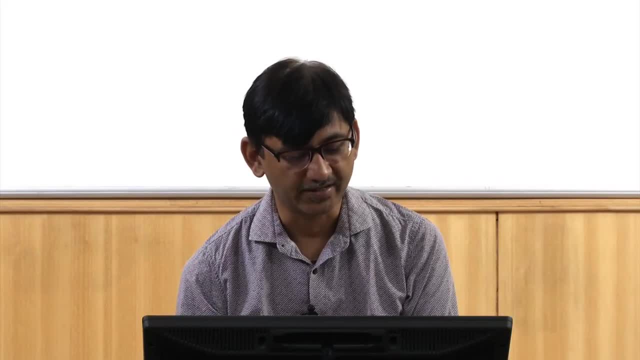 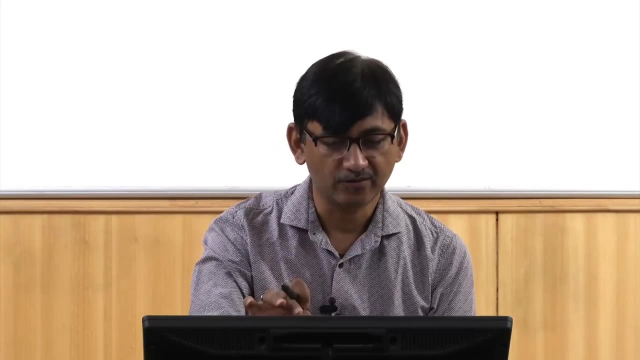 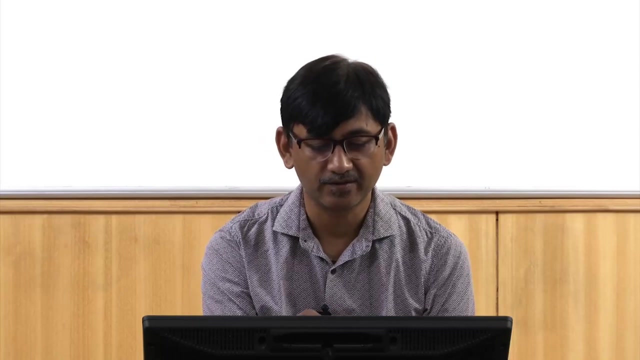 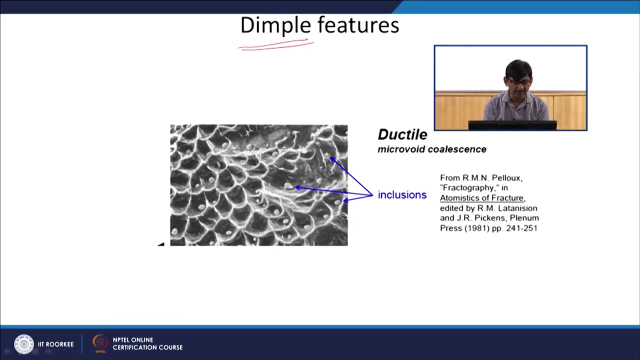 Okay, So this is how the whole deformation takes place. So now, because of this micro void formation and coalescence, Okay, The typical fracture feature which you see in ductile material is called dimples. Okay, So these are individual dimples and you can also see that there is a precipitate sitting. 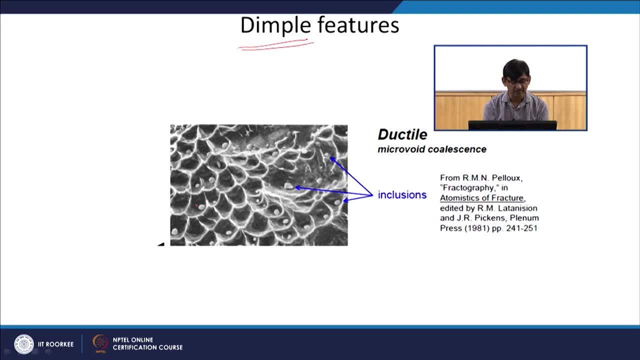 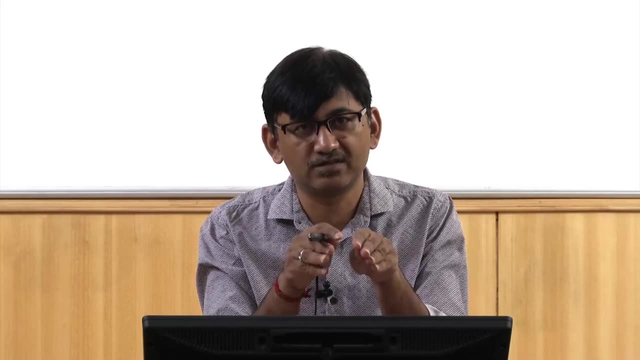 within the these dimples. that means that the micro void might have nucleated there. then it is. it was growing another micro void nucleated for this precipitate that is also growing and locally there is kind of a shear between the two of these holes. 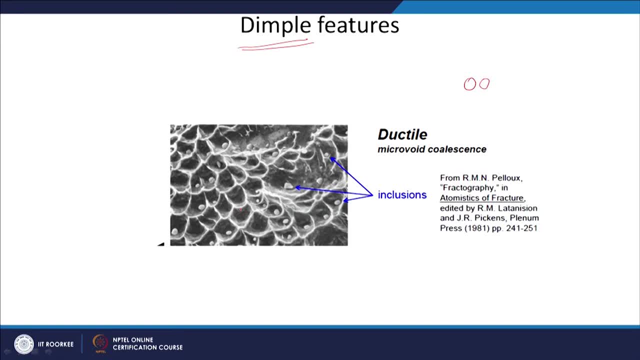 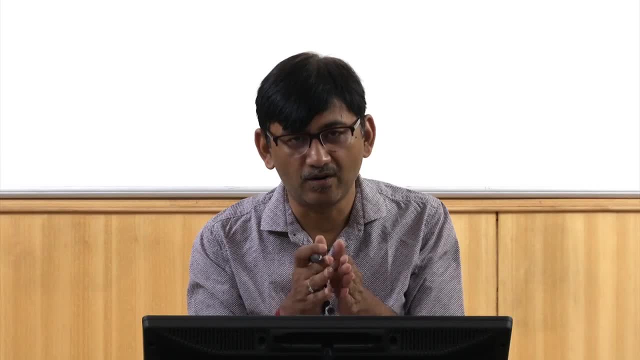 So you have one micro void like this, another micro void like this, Okay, And when the material is, whatever material is remaining between them, Okay, That is very thin, small volume of material that will shear out. So because of that, you get this raised portion here. 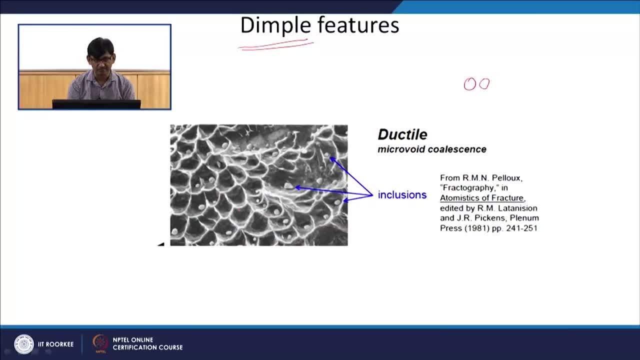 Okay, So this is a typical dimple fracture. So if it is under tensile mode, simple tensile mode, then it will look like a equiaxed dimples. Suppose the same thing is failing under shear mode, Okay, Which we see in cup and cone at the, at the extremities of the sample. 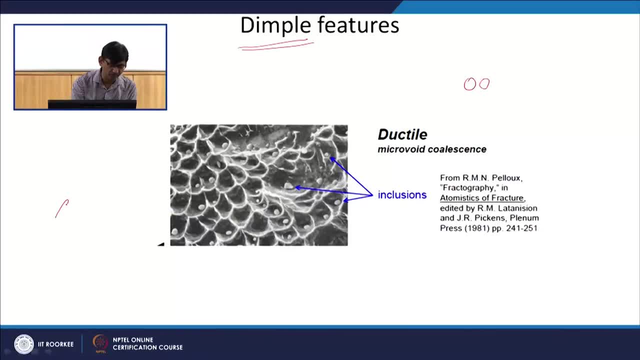 Okay, So this same dimples will, under shear mode, will get elongated. So it will look like this: Okay, So instead of equiaxed, you will get a elongated dimples. Okay, Elongated dimples when you have a shear mode. 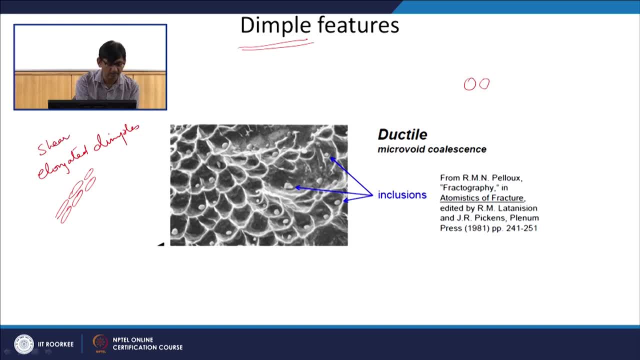 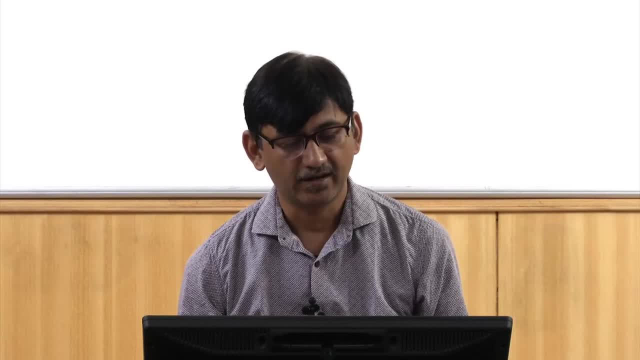 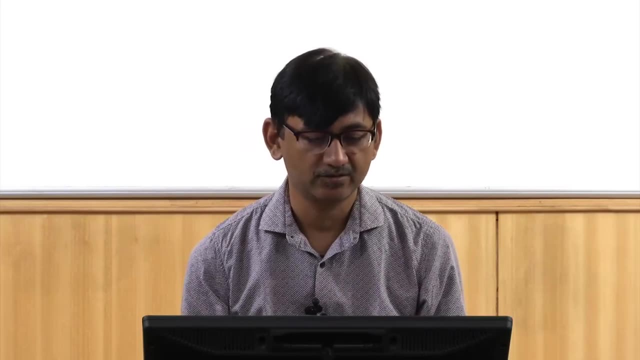 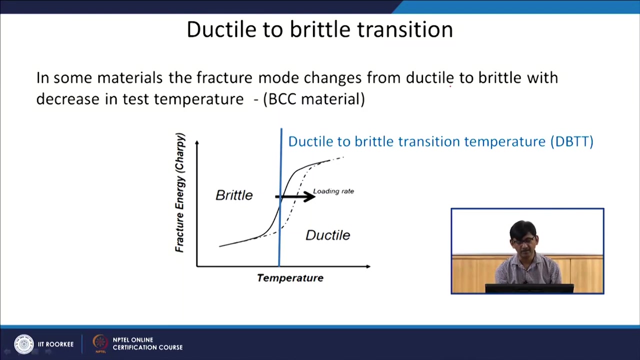 Okay. Okay. Now there is another problem with few materials, and that is that they behave different under different mode at different temperature. Okay, So this is what we call as ductile to brittle transition. So in some material the fracture mode changes from ductile to brittle with decrease in temperature. 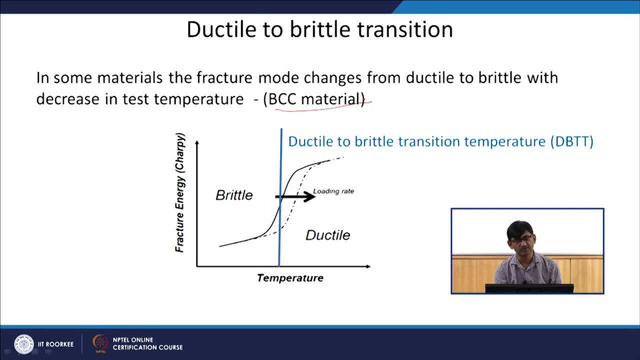 And especially BCC materials, are susceptible to this. Okay, So if you see the, this is fracture energy. that means how much energy is absorbed by material during the fracture process. So at high temperature it is behaving in a ductile manner. Okay, So ductile is always safe, for example, if I have any kind of impact. 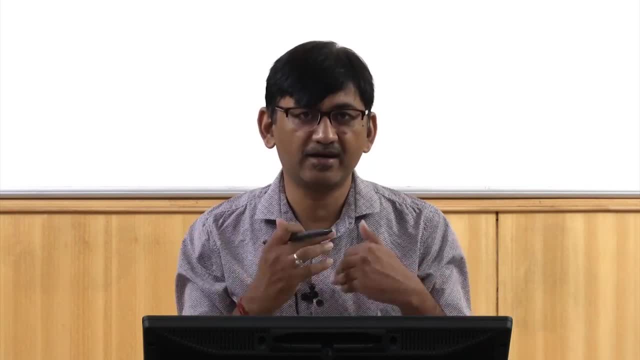 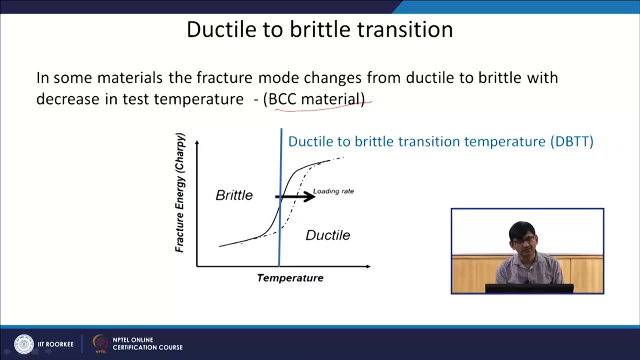 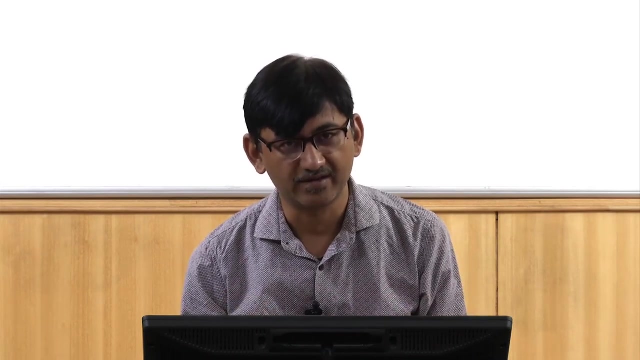 Okay, If it is a ductile material, it will only give a dent. Okay, It will not break into two parts. Okay, At low temperature it starts behaving as a brittle material. So now any impact on the structure it will. it may fracture into or there may be a initiation. 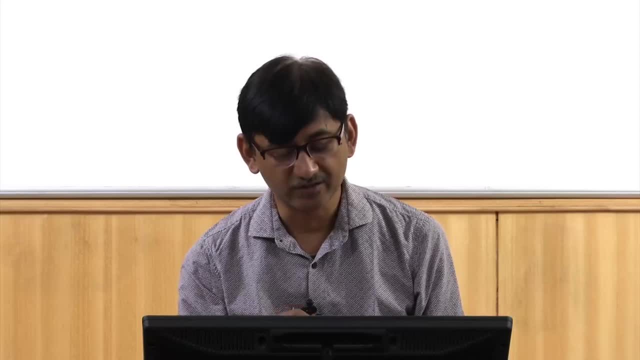 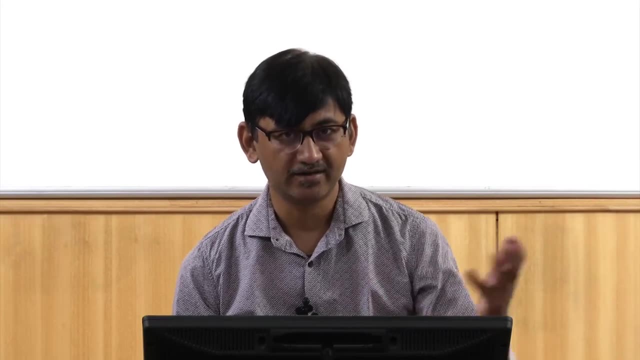 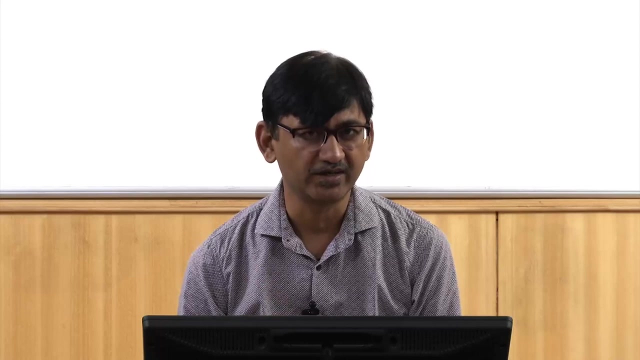 of crack. Okay, So with temperature, and that is what happened with the Titanic. Okay, Because the material which was used under the when it was going through the Atlantic Sea, Okay, Atlantic Sea, the temperatures, and I think it was winter, So the temperatures were low. 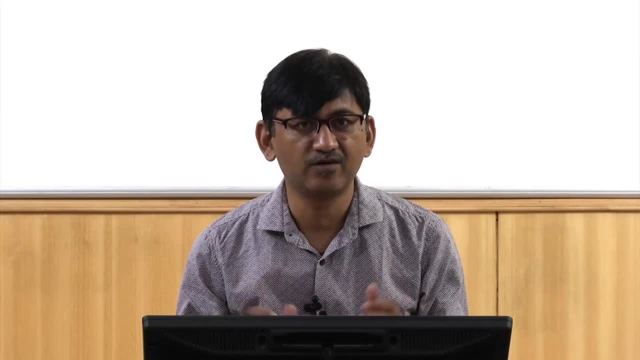 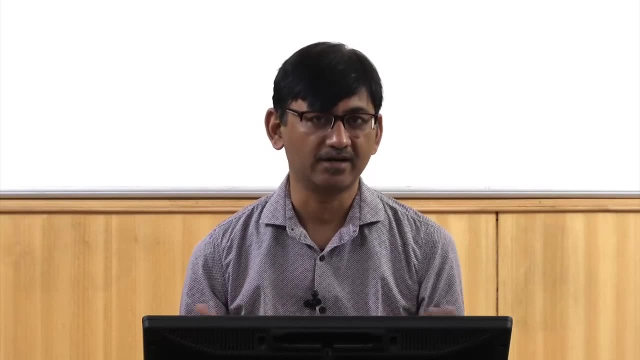 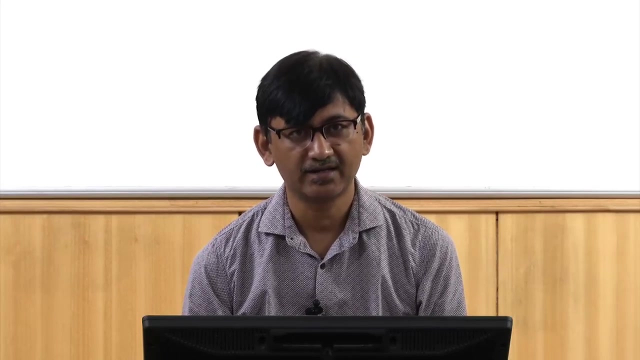 Okay. So in that temperature the material was behaving in a brittle manner. Okay, They might have done testing of this material, but they might have done testing at room temperature or little bit higher temperature. So there the material was behaving like a ductile material. 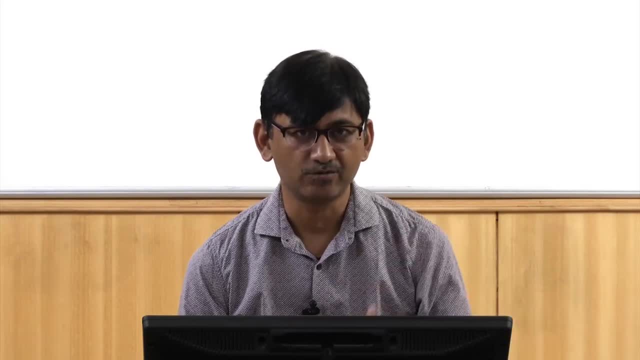 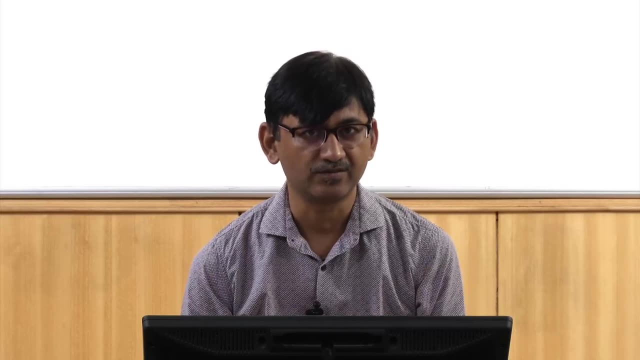 So they use that material, Okay. But when it went into the Atlantic Atlantic Sea, Okay. And when, because of in the night, Okay, Because of in the night, the temperatures of the water must be low, So at that temperature it started behaving like a brittle material. 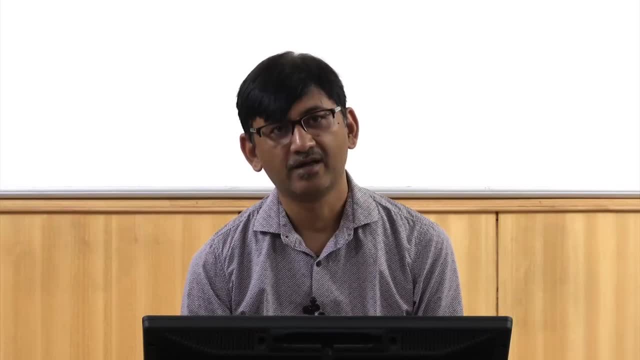 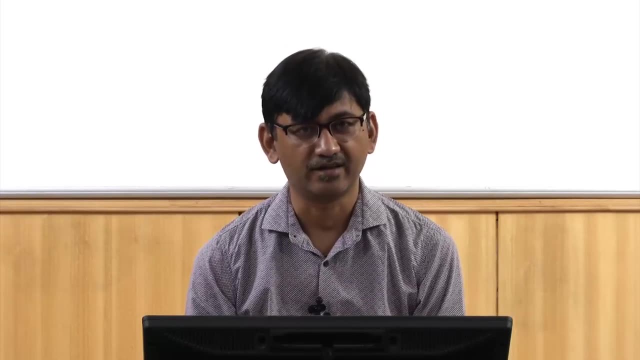 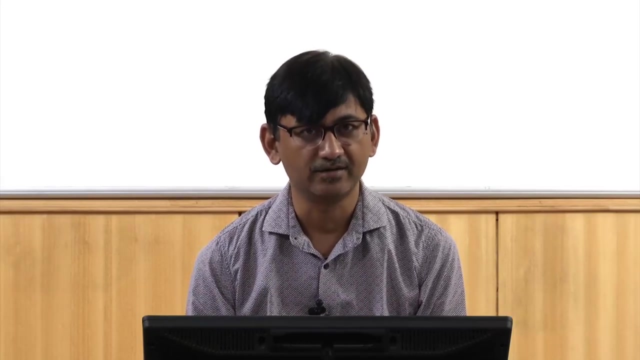 So the? when the iceberg hit the ship, Okay, It, instead of just giving it a dent, Okay, What it did is it is initiated. the crack in the in the structure of the ship, Okay, And that crack then started propagating, and then you had the, that accident. 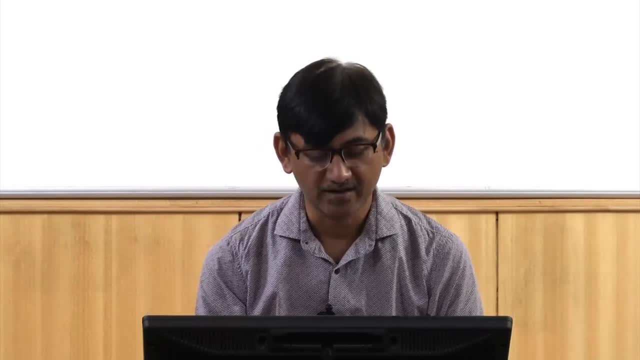 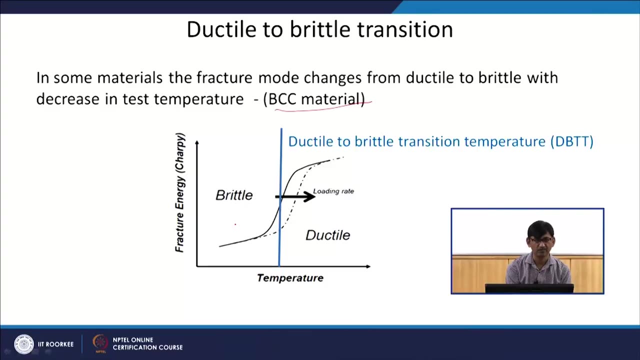 Okay, So now the then, of course, lot of material research took place. people took care of that problem. So at least they can bring the transition temperature to very low temperature, which are you will not find in under the service condition. Okay, So this kind of research keeps going on as you face some problem or other. 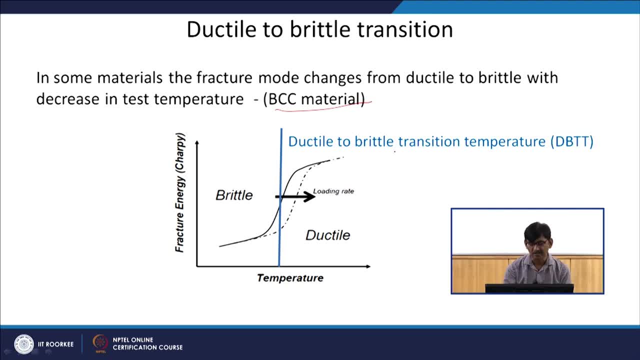 Okay, So the temperature at which this transition take place takes place is called ductile to brittle transition temperature, DBTT. Okay, So basically we have to take care of DBTT for any material. So when you develop a new material, we you have to do testing at room temperature high. 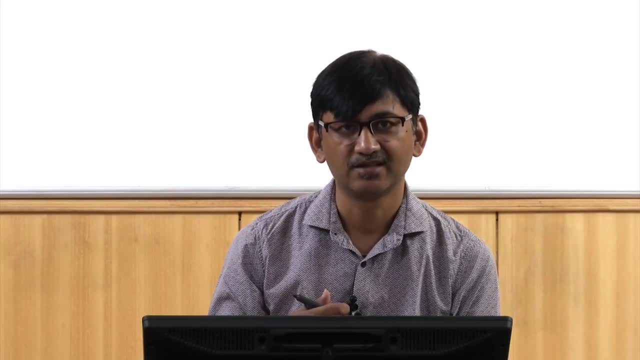 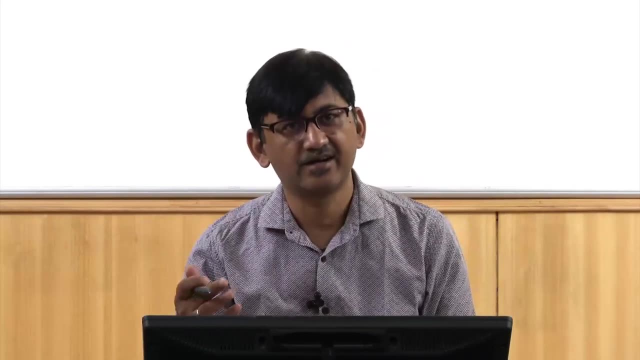 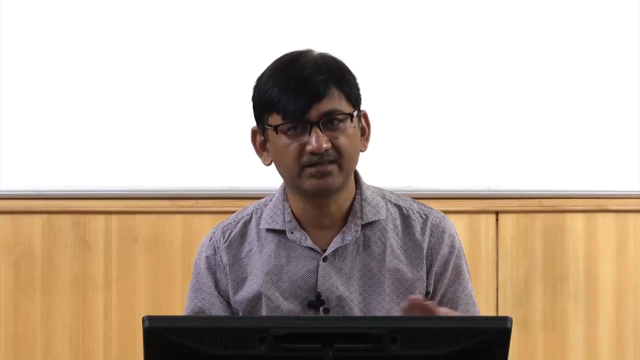 temperature: low temperature under different loading conditions. static, low, quasi static loading means at very slow strain rate, high strain rate testing, which we call as impact. Okay, So we can, depending upon the application, if it is not going to see any high temperature, we will not do any high temperature testing of that. 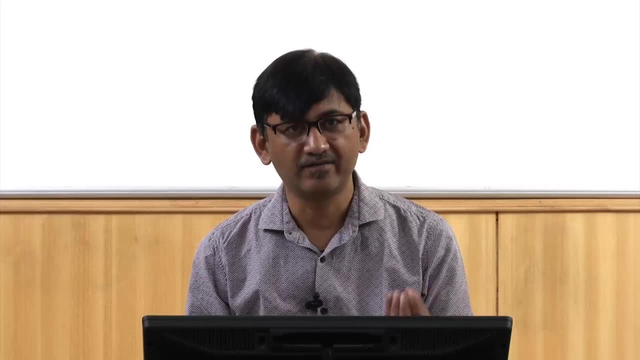 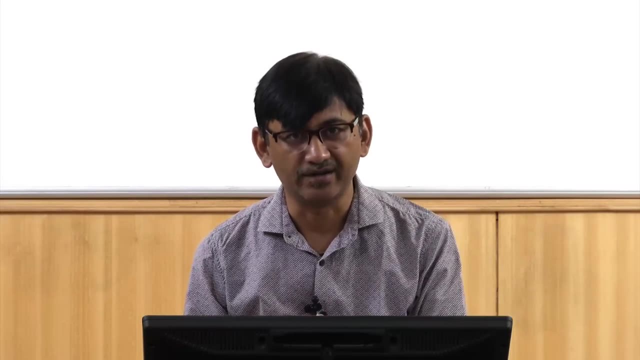 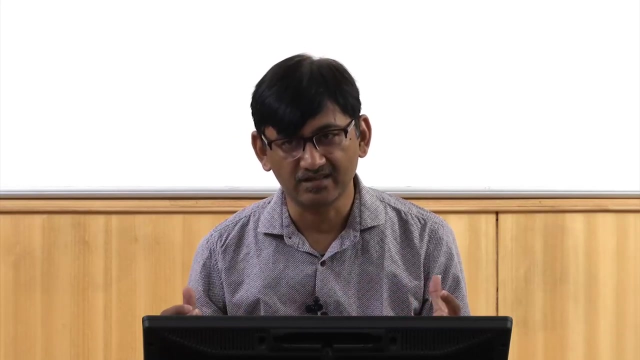 But suppose you are developing an automobile material. Okay, I will test it under quasi static condition to design the structure. but I will also test under impact loading. Okay, Because under the crash condition there should not be any fracture in the sense that it will. 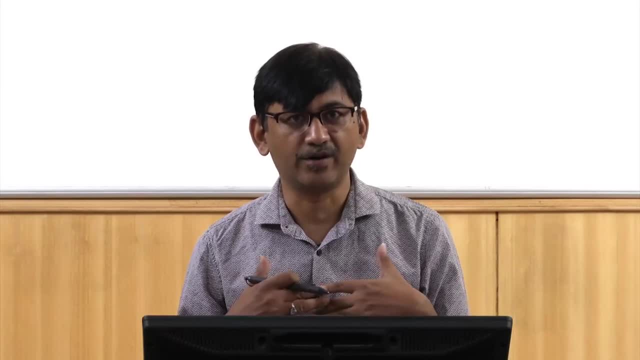 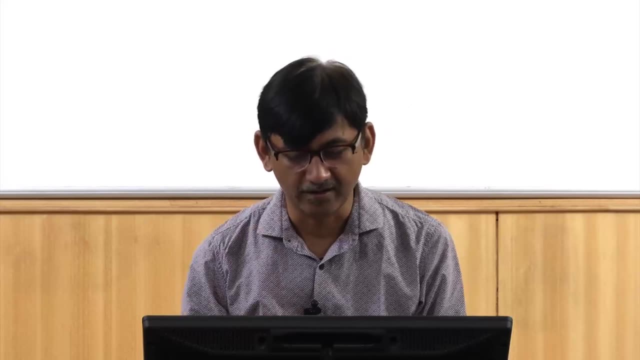 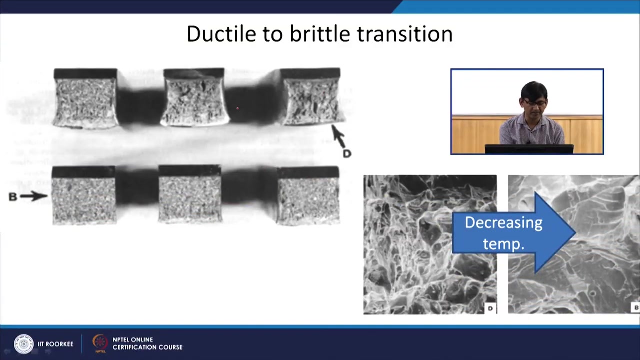 fracture like a brittle material. I want to it to absorb maximum energy by deforming plastically. Okay, And that is what we will see in the next slide. Okay, So this is the ductile to brittle transition. So the sample tested at different temperatures. so at high temperature it behaves like a ductile. 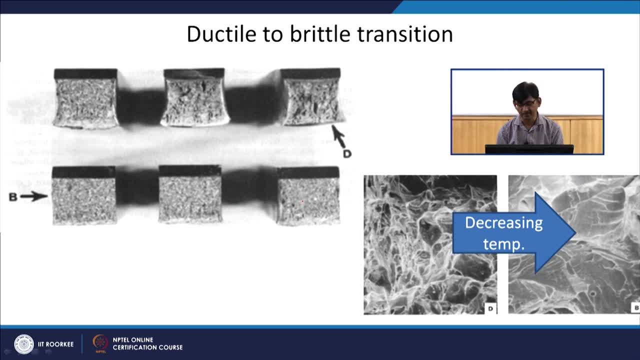 material and at low temperature it behaves like a brittle material and the fracture morphology also changes, So as a function of decreasing temperature. So here you can see that it has a ductile, fibrous kind of appearance, whereas in this case you have faceted and river markings are there. 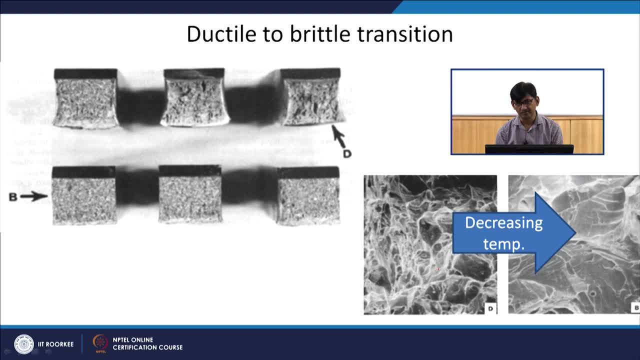 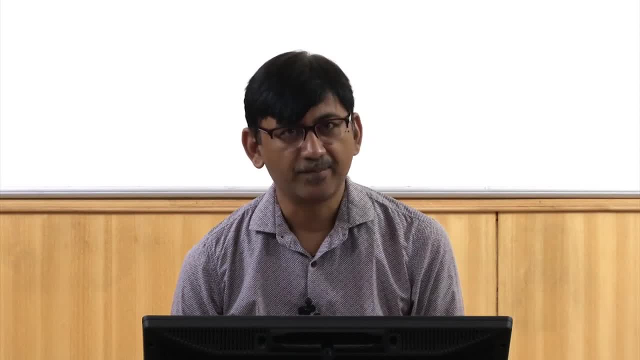 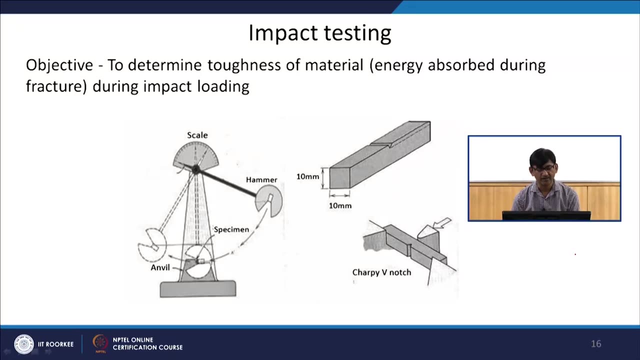 So for the same material, the fracture morphology has changed from ductile to brittle. Okay, Now, this is just one slide on the impact testing. that is one of the important aspect of any material development, Especially for automobile, as I was telling you. Okay. 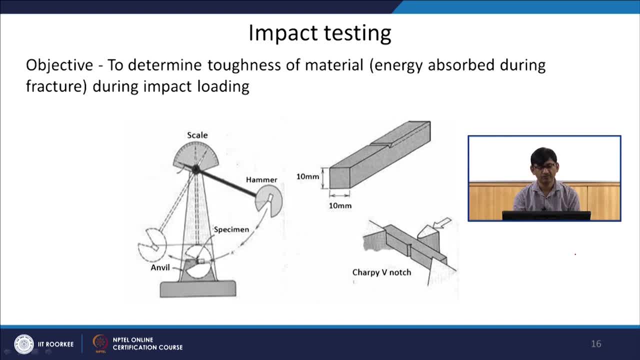 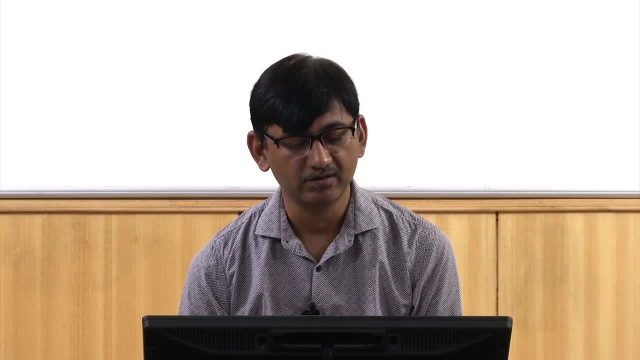 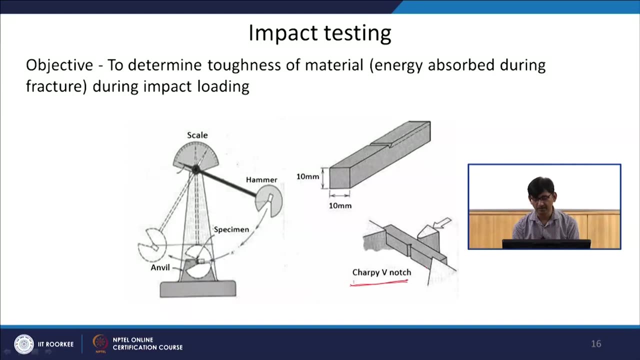 So basically, our objective here is to find out what is the energy absorbed during the fracture. Okay, So maximum energy absorbed is what we want. Okay, So there is one type of test which is called Charpy V notch test. Okay, And this is the arrangement for the atom. you create a pre crack kind of condition already. 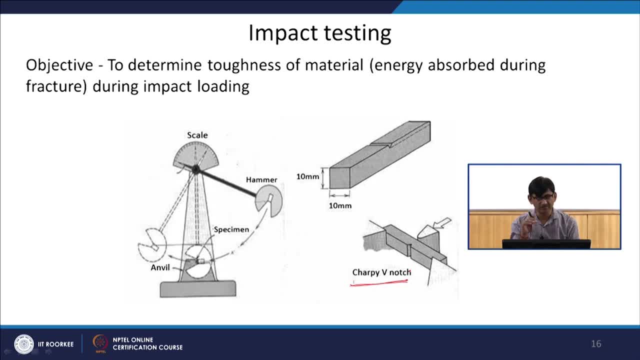 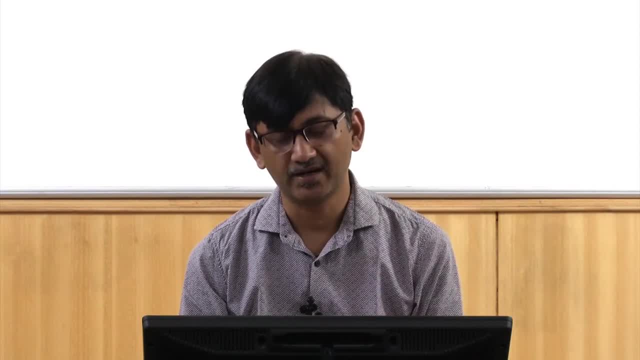 here by providing a notch here, So that the stress will be concentrated in this region only. Okay, So you are kind of trying to simulate that already there are flaws present in the material and if you have a impact loading, how much stress it is going to absorb. 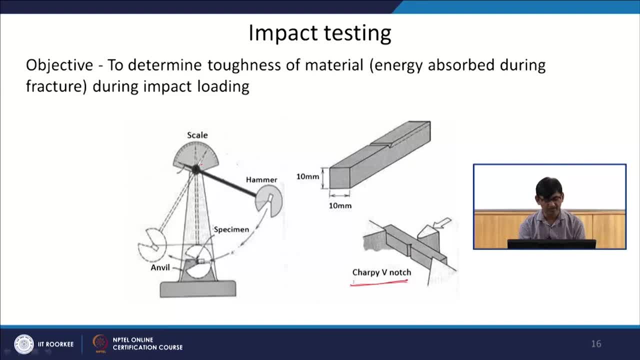 Okay So, and to do the test, a very simple apparatus is there. so you have a very high hammer with lot of weight is there. you take it to certain height, so now it has some potential energy, and then you remove that. Okay, So that it take a swing here, so that potential energy will convert into kinetic energy. 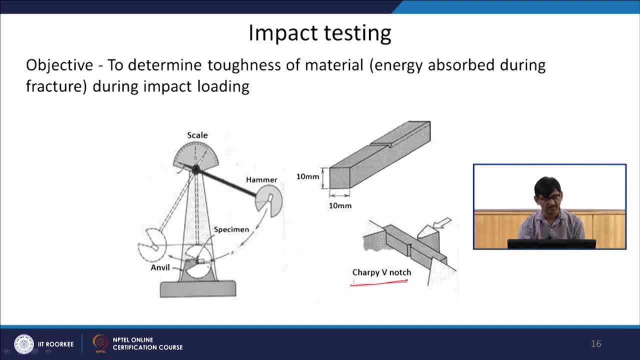 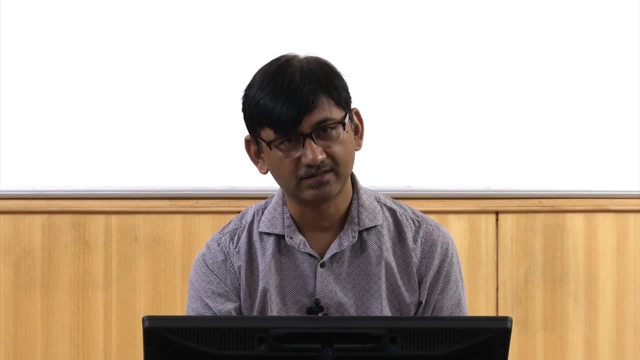 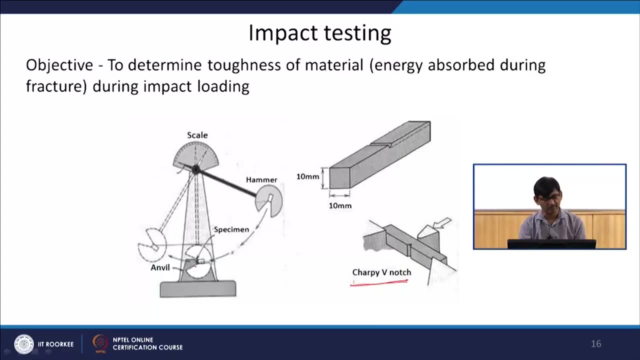 So at this point you will, it will have maximum kinetic energy and it will hit the sample and then it will go on the other side. So whatever is energy absorbed in this fracture of this sample, Okay, That much less energy will be there for it to swing to certain height.